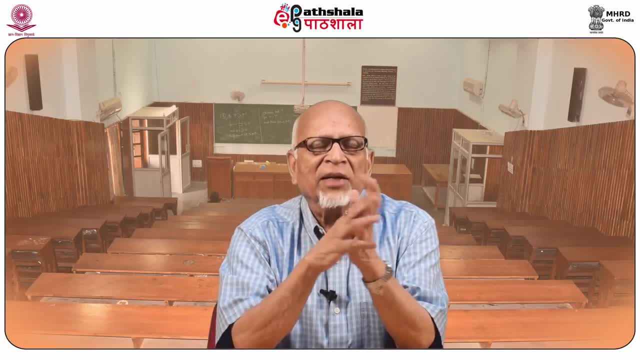 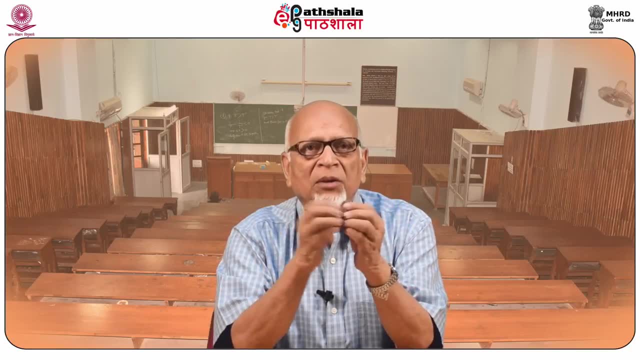 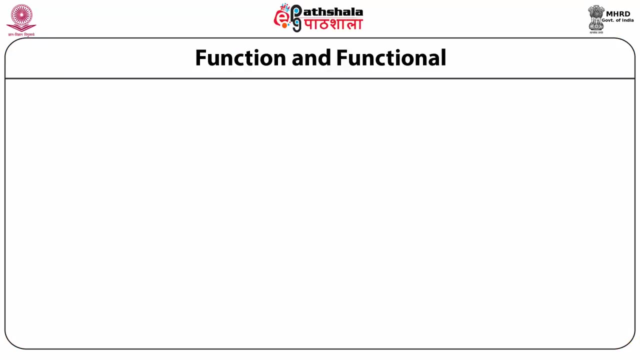 the Bernoulli brothers by Euler, Legendre, Lagrange, Hamilton and Jacobi, to name a few important contributors during the 18th and the early 19th century. definition of functions and functional. You all know that a function f of x is defined. 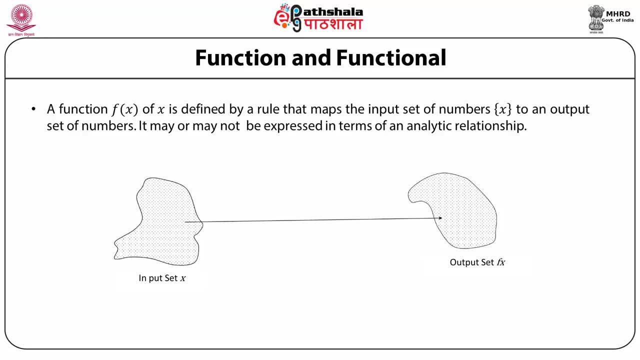 by a rule that maps the input set of numbers given by the set x to an output set of numbers. It may or may not be expressed in terms of analytical relationship. There could be any relationship which maps one number in the input set to a corresponding number in the 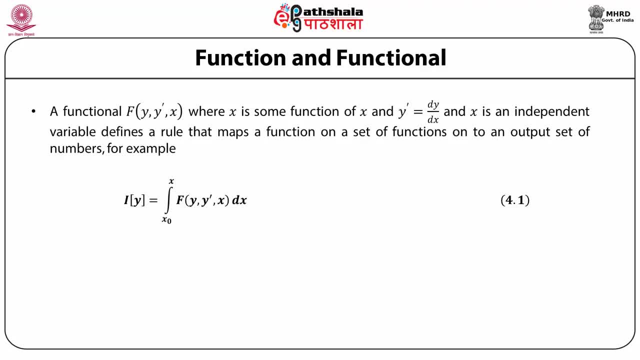 output set. A functional, on the other hand, represented is capital F of y, y prime and x, where y is some function of x and y prime is equal to dy by dx, and x is here an independent variable. Now this functional defines a rule that maps a function on a set of functions onto an output. 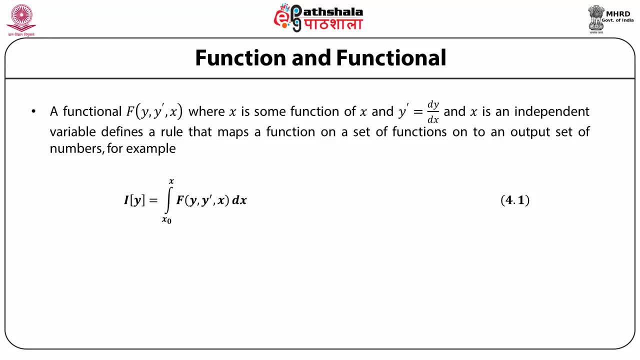 set of numbers. For example, if we consider this integral i of y, which is an integral between two points, x naught and x, of an integral of a function of y, y prime and x integral dx, Then this quantity i of y is a functional where the integral f, y, y prime, x is a simple. 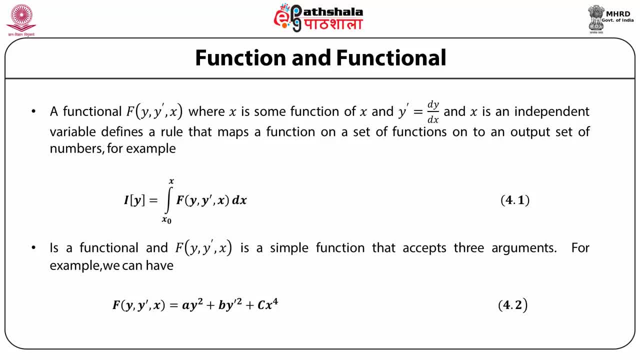 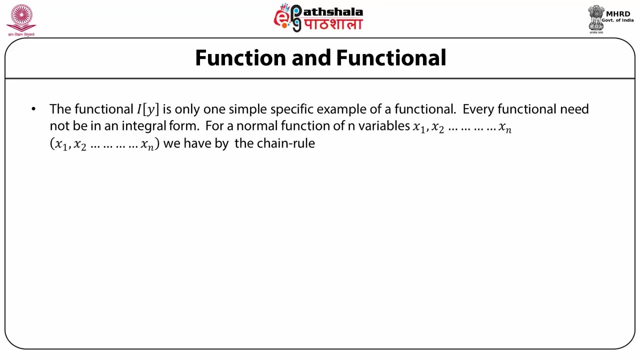 function of three arguments: y, y prime and independent variable x. For example, we can have for this integral f, y, y prime, x as a y square plus b, y prime square plus c, x4, etc. the functional i of y. the way we have given is only one simple, specific example of a functional. 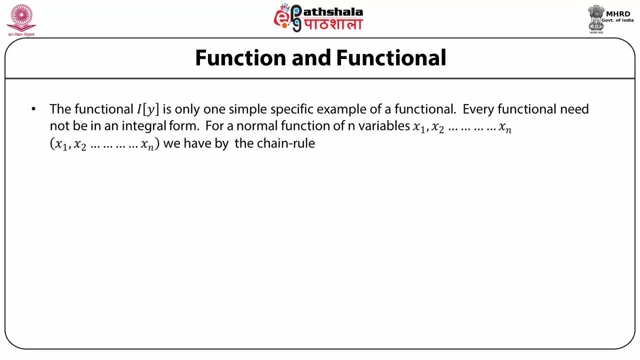 every functional need not be given in an integral form. remember that for a normal function of n variables, that if a function f of n variables x1, x2, xn, then from the chain rule we have the differential of the function f is equal to df by dx1 delta x1 plus df by dx2 delta x2. 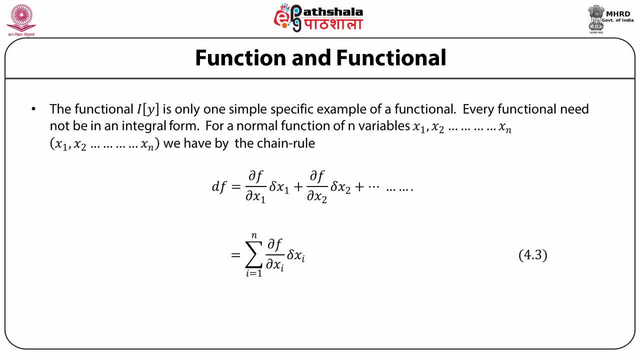 and so on and so forth, till df by dxn, delta xn, which can be written as sigma partial derivative f with respect to xi, into delta xi, sum over all xi's. this is for a function. now we have a similar form for the variation of a functional. 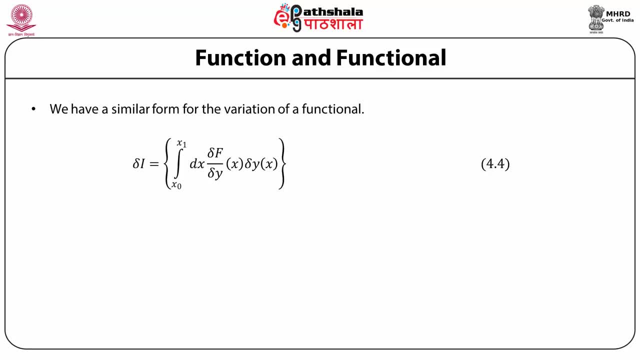 so our functional delta i is our function. functional is i and the variation of this functional delta i is equal to an integral from x0 to x1, over dx of the variation on the function f with respect to a variation on y into delta y of x, with delta f by delta y is equal to delta f by delta y. 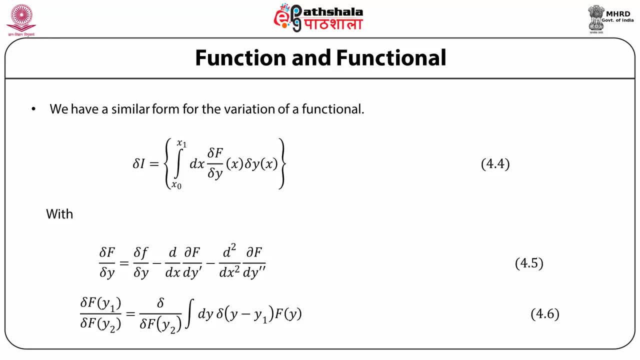 minus delta f by delta y applied to the function f master. f times the series a radical times the function of a function f of this double invariant function. so this is the nothing is exactly something of an feminist. d y, delta y minus y 1 f y. this is how it is defined. so with this we can prove the following: 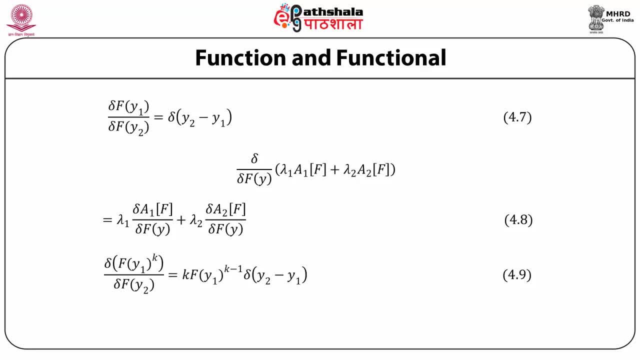 results. first is that delta f y 1 divided by delta f y 2 is simply a delta function of delta y 2 minus y 1 and delta delta f y of a linear combination of two functions of this function: f, that is lambda 1, or multiplied by a 1 of f plus lambda 2, a 2 or f is given by lambda 1 of delta a. 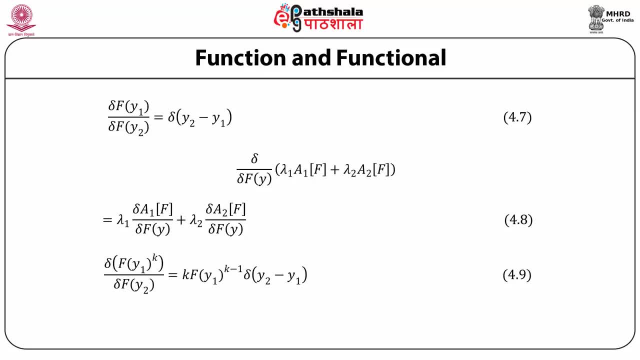 by delta f plus lambda 2 multiplied by delta a, 2 by delta f. and another property is that delta delta f? y2 of the kth power of f? y1 is k times the function f? y1 to the power k minus 1, into. 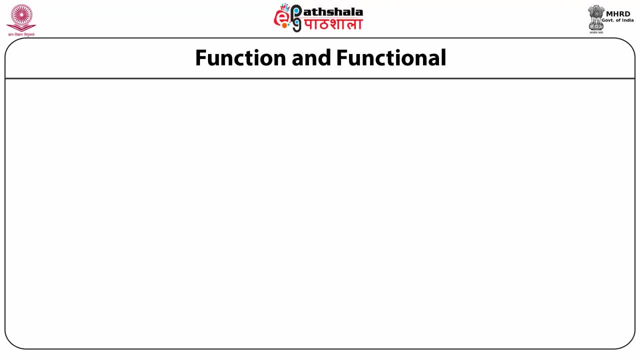 the delta function of y1 minus y2.. Now delta delta f2 of d y1. we can see that this is so delta delta f of y2 of the integral d y1 sigma over k, a, k, y1, f, y1, k is equal to d y1 delta y1. 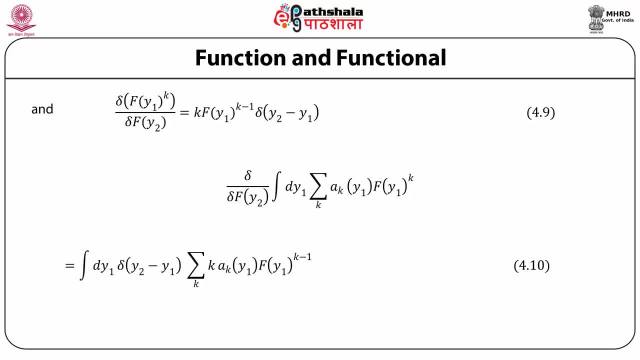 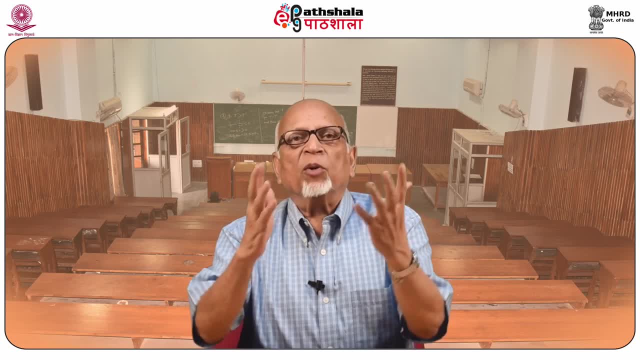 by y2 into sigma, over k, a, k, y1, f, y1, k minus 1.. So this is another property of the function. So let us start with the calculus of variations. What is the problem here? What is the problem which we want to solve? See in the calculus of variation. the problem is to determine a function f of x such that if you consider the integral j over dx from some two fixed points- x1 and x2- of a function f, which in turn is a function of y and remember, the y itself is a function of x. So f is a function of y and is a function of y prime. 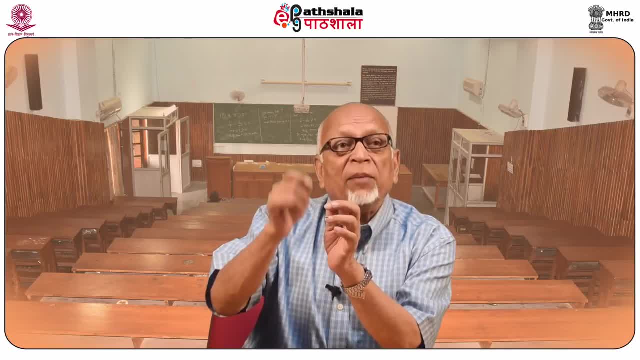 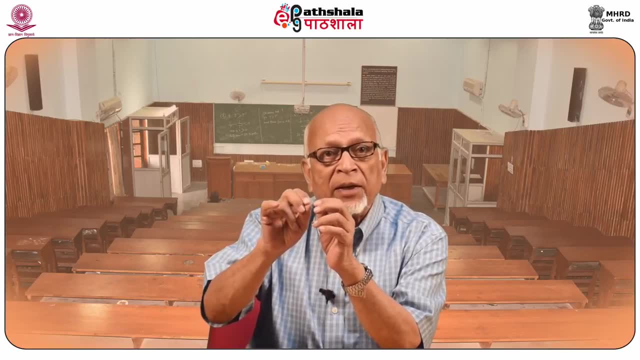 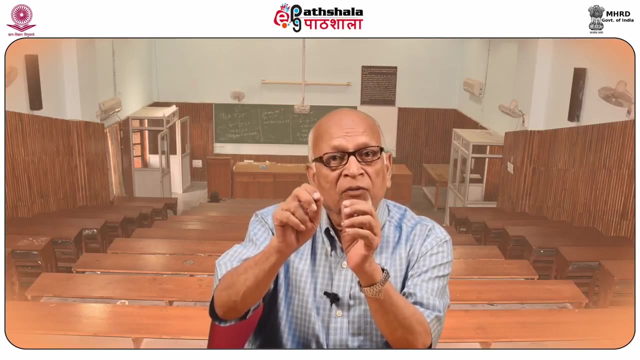 So y prime. by y prime we mean dy, by dx, the derivative of y with respect to x and x, So x here is an independent parameter. So this is an integral which occurs in many physical problems which we want to Extremize, That is, we want 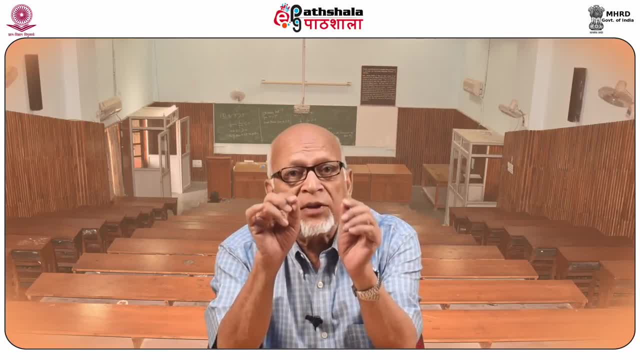 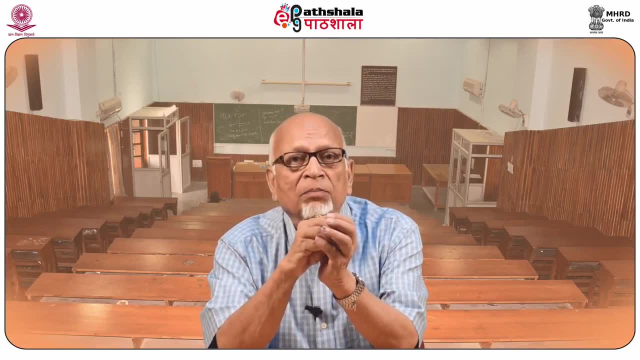 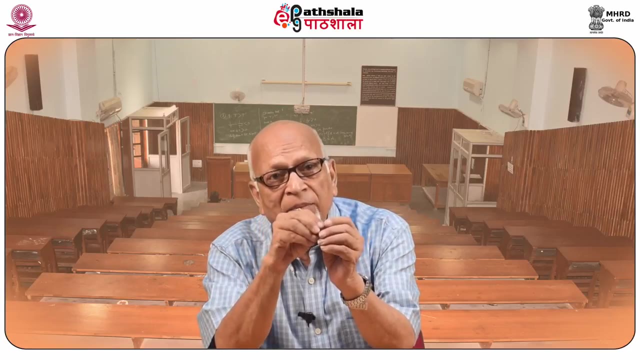 extremum value of this integral. By extremum value we mean that the value could be either a minimum or a maximum In the above equation. remember that y2 is the function of x and y. prime is dy by dx and x is an independent variable. 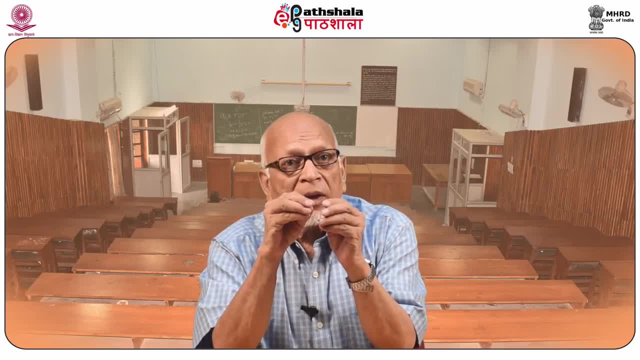 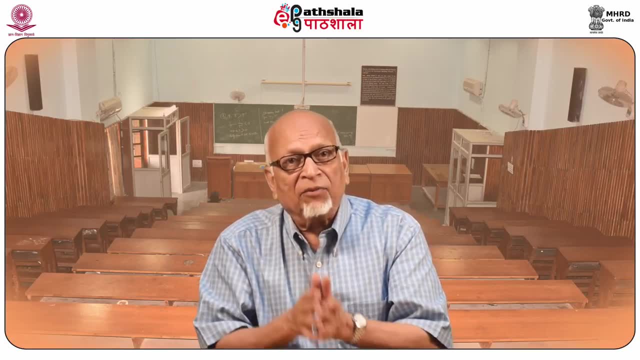 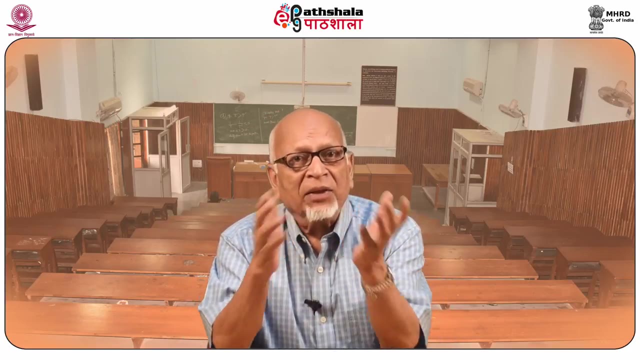 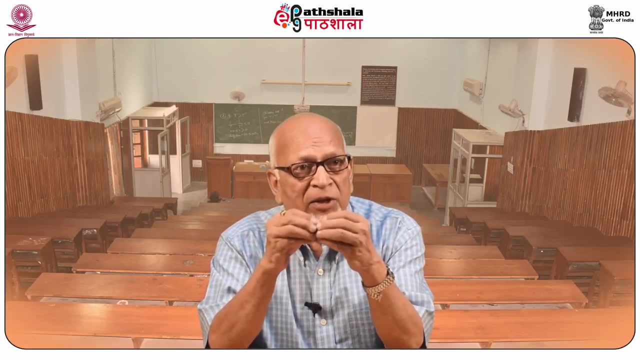 The function. f, in fact, is a function of the functions, because f is a function of yx and y, prime x and x. This is called a functional and is given and is again to you. So you have, we have to extremize it and the limits of the integration are fixed. 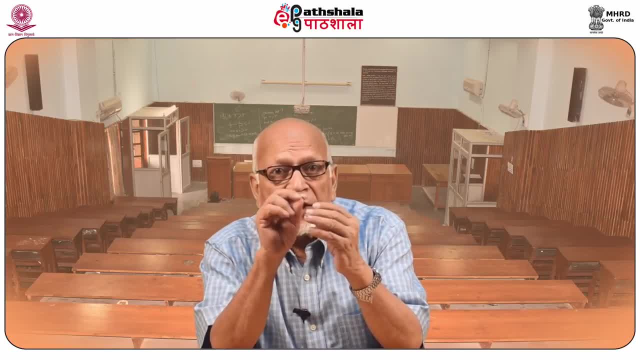 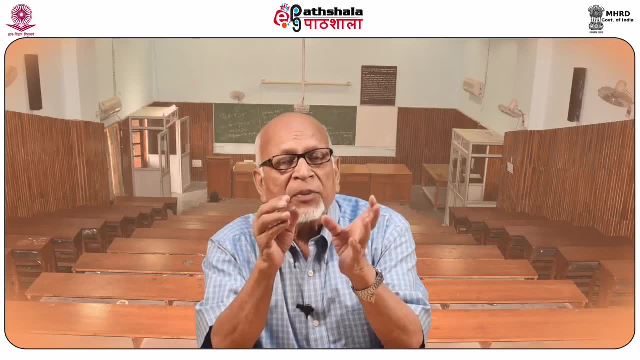 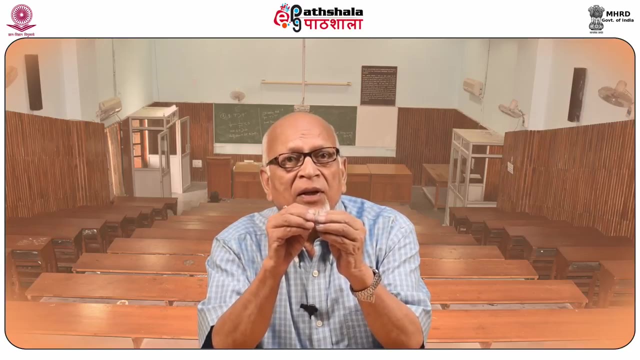 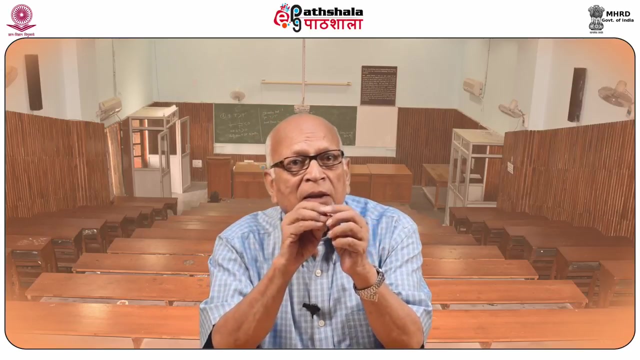 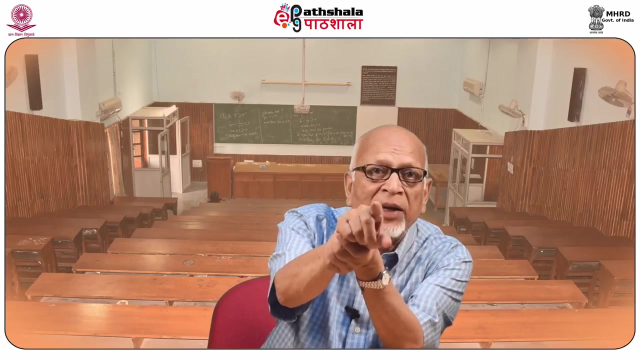 This function is is varied until an extremum value of j is found. What does it mean? This means that if a function y of x gives integral j a minimum value, then see the functional f depends on y and y prime, but y prime is just the derivative of y. 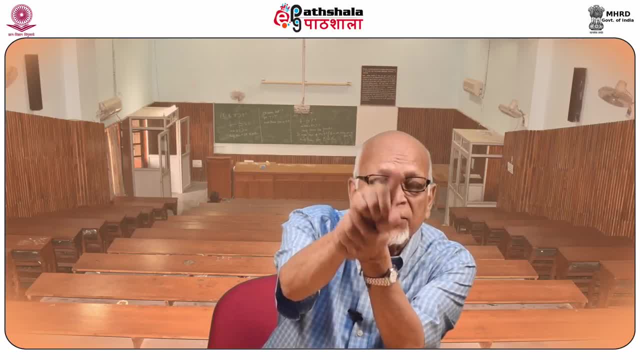 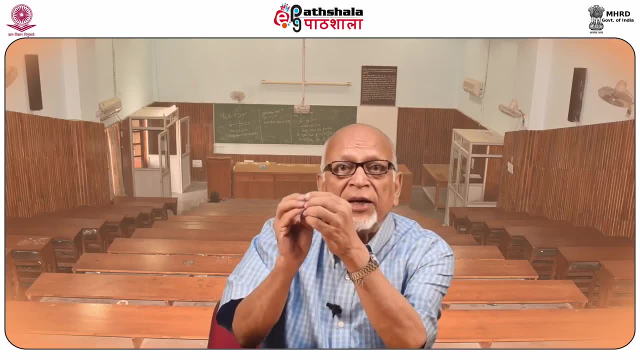 So if we can find a function y which makes that integral j a minimum value, Then it means that if we ticket the neighboring function close to y, then this must result either an incredible or a decrease in j, if j is extremum, If j is minimi. 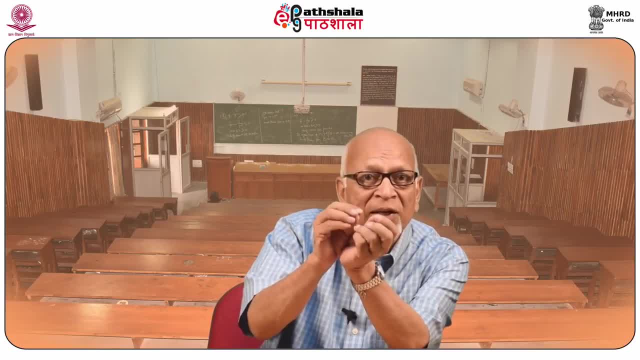 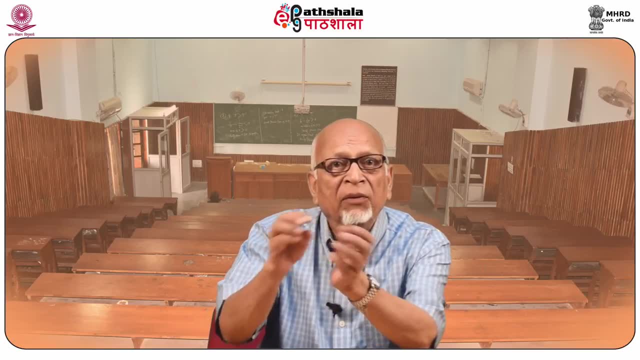 than it means that If J or j is extreme, if j is minimum, then it means that any neighboring function which draws, Then this should be checked, So So, So then it should be filled, So Then it should be filled. Here it should be filled. Panther has to get present to set number two. Then it can be used as a function of n equals n plus 1, minus outcome capital would be deshalbioettes. So you see here that this for each nowadays. 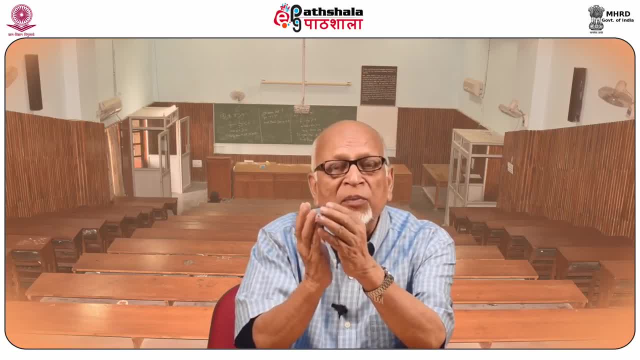 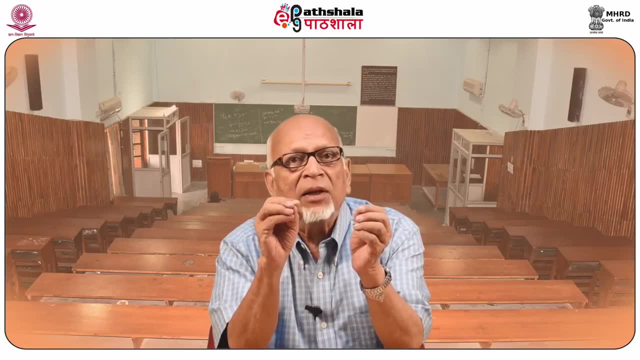 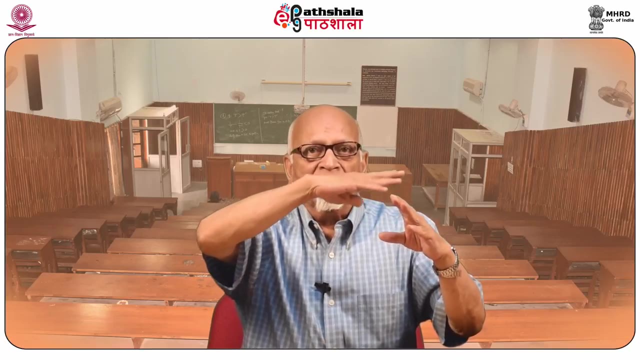 Minimal. lucky would be that Adams had a function which draws a minus 1 index. is point's wise a benefit to it? function to yx will increase j, so let us represent all possible functions yx. so there is a function yx which extremizes the integral. so let us consider all possible functions y of x by. 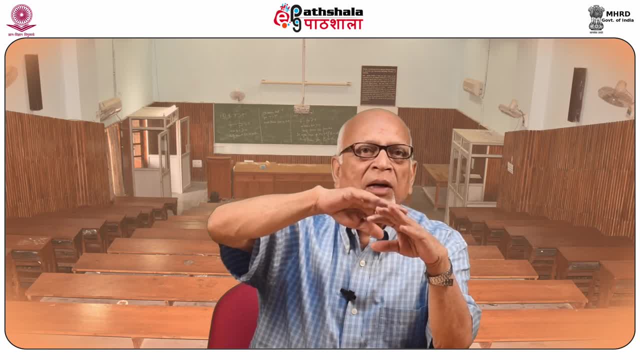 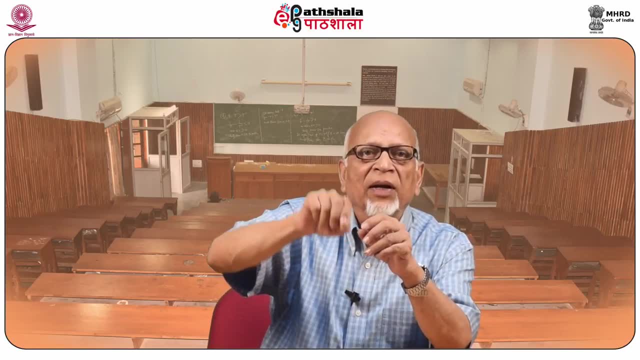 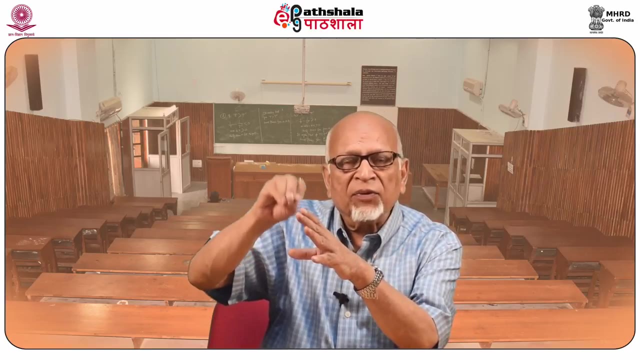 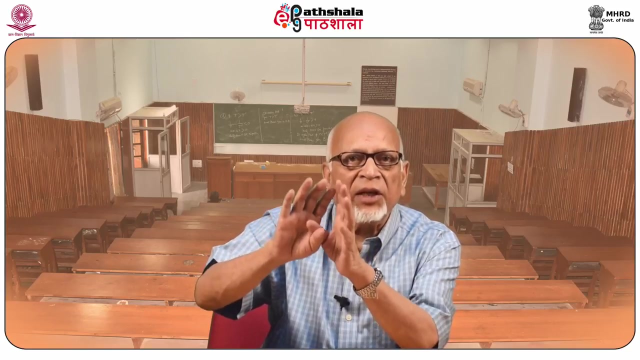 a parametric representation that any function y is given is a function of some parameter- alpha and x- such that when alpha is equal to zero, then y, which is a function of now x alone, is the function that will extremize j. in that case we can write this function: 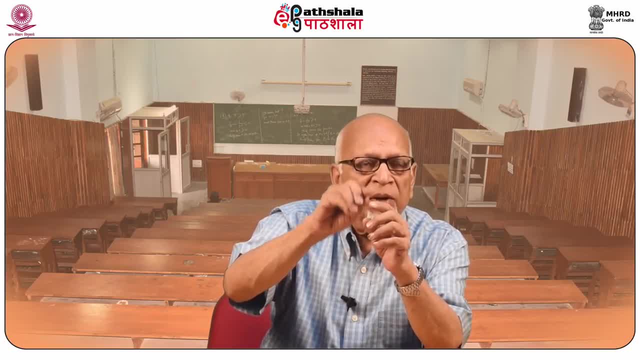 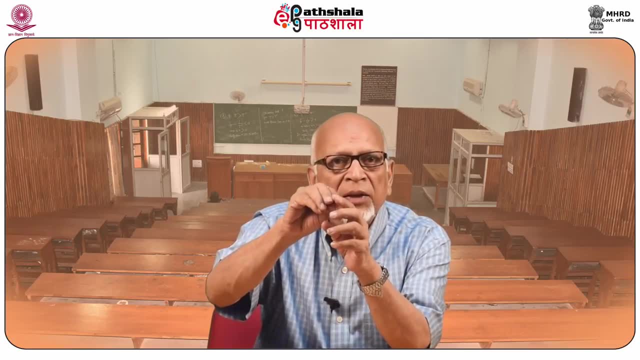 now x is the function that will extremize j. in that case, we can write this function, y, which is a function now of the parameter alpha, which we have introduced, and the independent variable x as equal to y, a function when alpha is equal to zero and x that is the function. 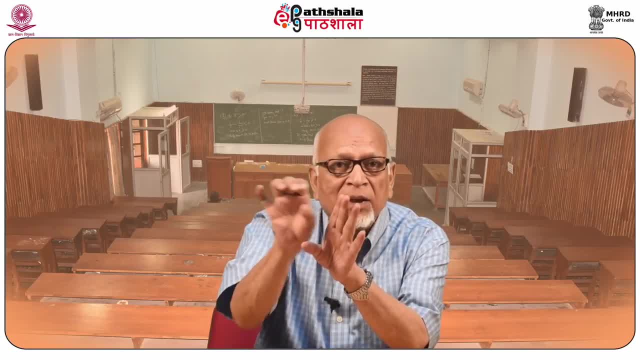 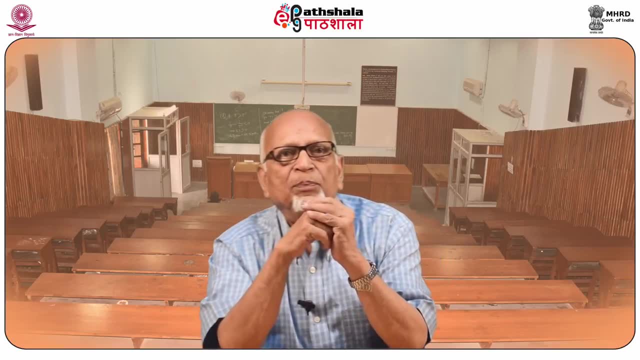 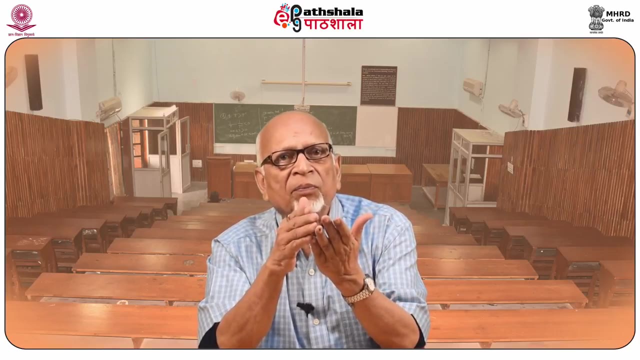 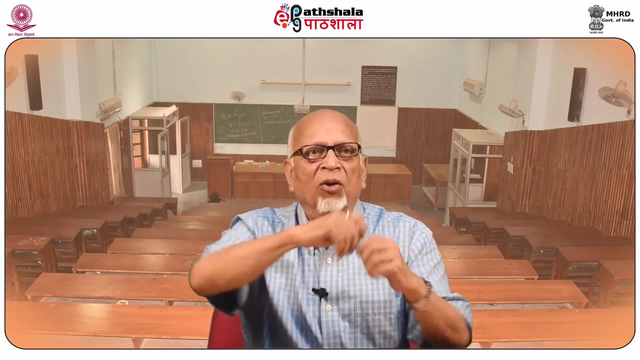 which extremizes the integral, plus a small variation parameter by alpha, which we have written as alpha, eta x, where eta x is some function of x which has continuous first derivative and which vanishes at the end points. because all the neighboring paths that we take, they bring functions, they should all end at the same. 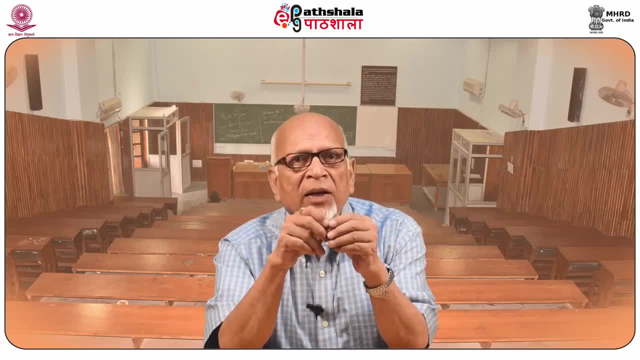 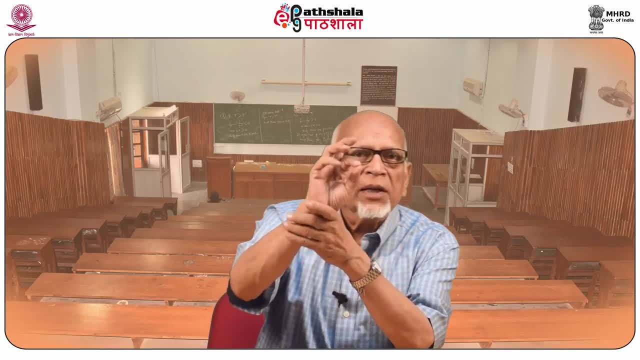 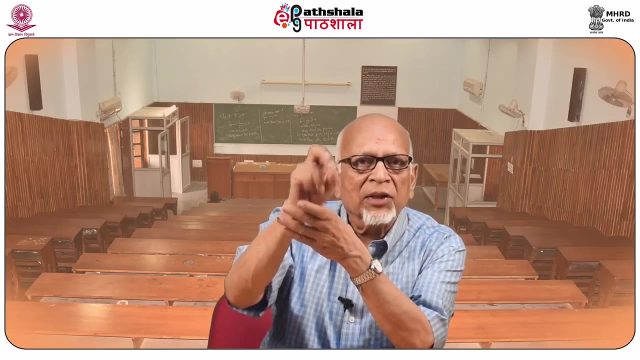 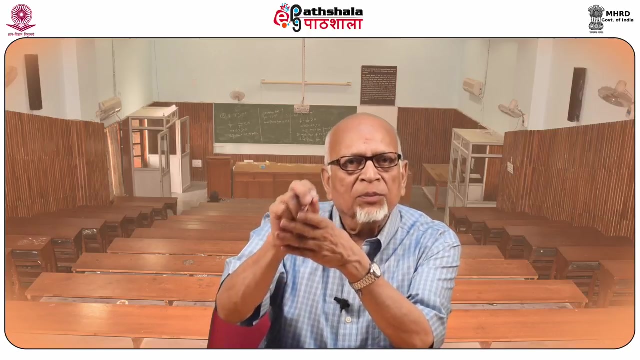 points x one and x two, since y, alpha, x, yx at the end points of the path. so that means this eta function, the function eta evaluated at the end point x one is equal to the function eta evaluated at the point x 2 and must be equal to 0.. The integral j now becomes a function. 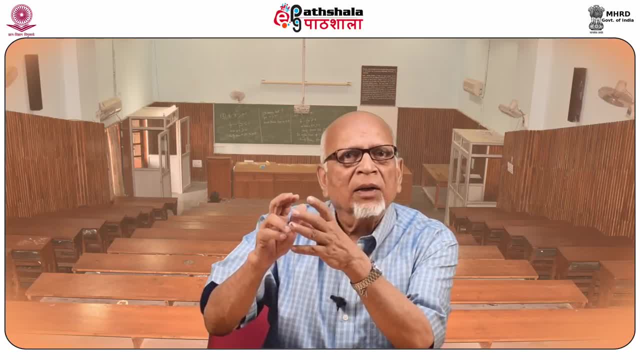 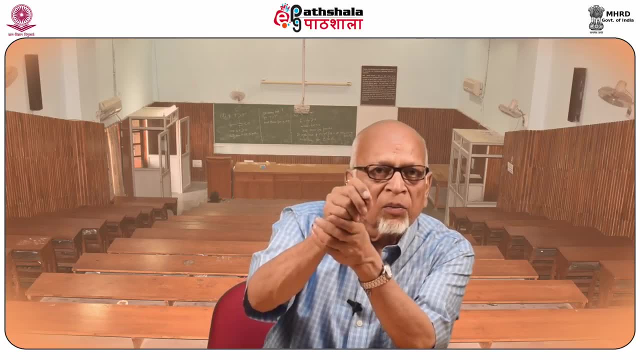 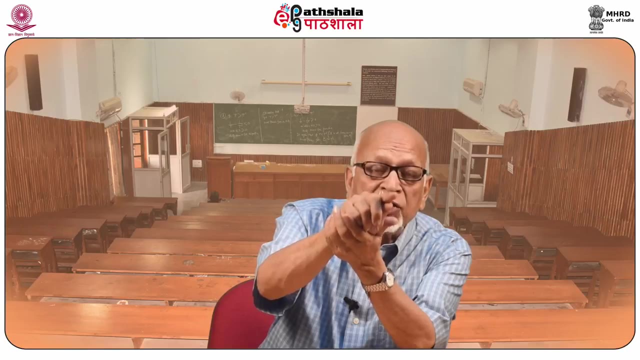 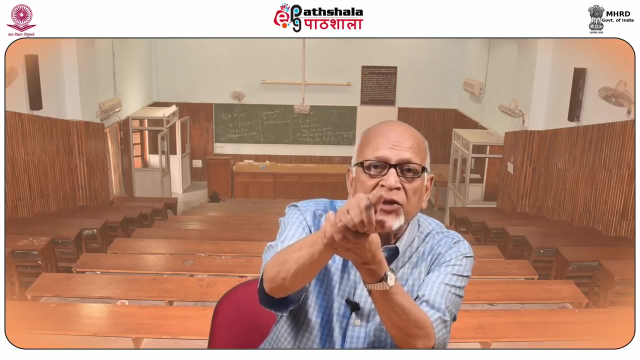 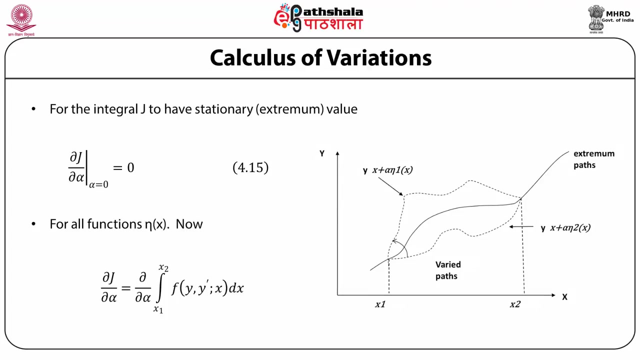 of alpha and, of course, eta's. So this j? x can now be written as a function of f, of a function which depends on the function y, which is a function of alpha x, y dash, which is a function of alpha x and x. Now we have considered the integral j, which is a function 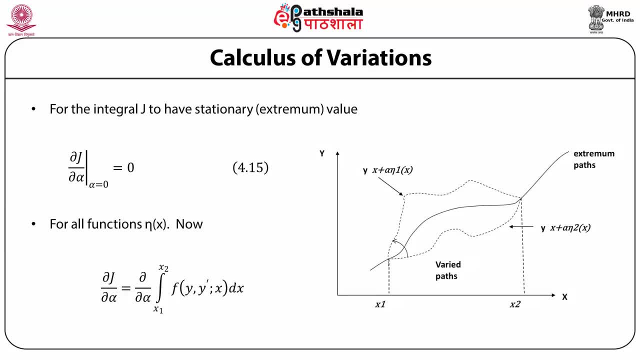 of alpha and we want to extremize it. Now, if you look at the diagram shown here, we have shown the path by solid line, which is the extremum path, which means on this path J is an extremum or either a maximum or a minimal, To see the variation of J over: 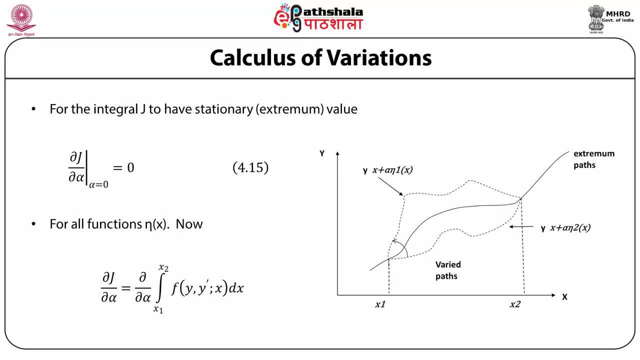 the nearby paths. let us consider two vari able paths, one below this and one above this, and we have shown this. vari able paths be given by extremum path y, plus some perimeter times, a small variation, eta 2, And another path which means a plus or minus some parameterx, the donde and the other Yang D is seen as the vari able paths. 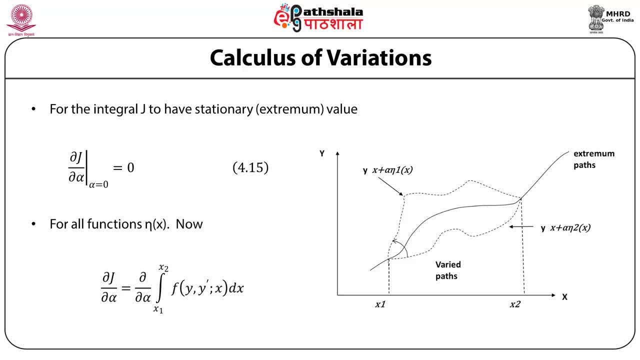 that be given by the extremum path, x, and the other엔 y plus some perimeter times, a small variation, eta 2, And another path is the Yu and U to the다가 wtheě given by y of x plus alpha times, eta1 of x when we are extremizing the path. 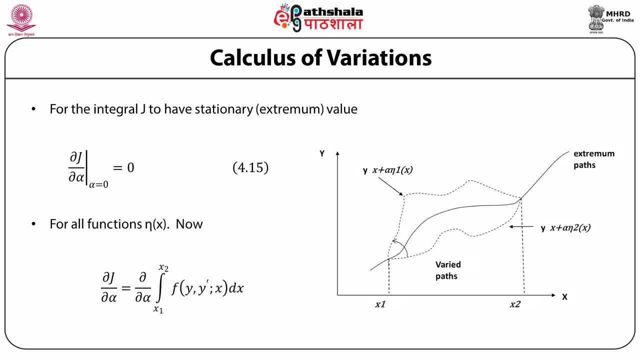 remember that the initial and final points are fixed, so x1 and x2 are fixed. so we vary the paths around the extremum path and then demand that the integral G takes up the extremum value, that is, the variation of J with respect to alpha. as alpha goes to 0 is equal to 0 for all functions. eta x, now DJ by D, alpha is DD. 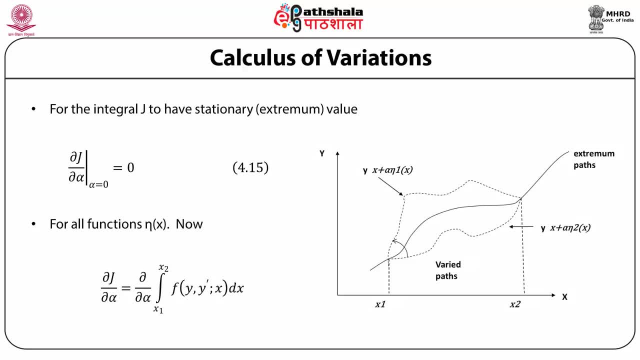 alpha of the integral from x1 to x2 of of a function, y, y, prime and X, DX, which is to be extremized, now DJ, by D alpha by differentiating given in the previous equation, as DD alpha of integral x1 to x2, f, y, y, prime, x DX is equal to the integral from x1 to x2 of the variation. 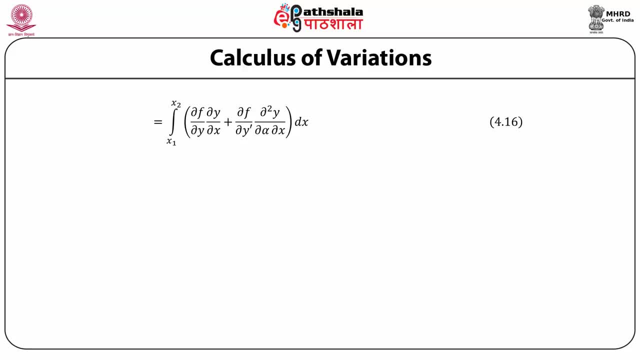 of f with respect to y into dy by DX, plus variation of f with respect to y prime and D to y by D alpha DX into DX. now the second term can be integrated by parts, so we can write the DF, dy, prime into D, DX of dy by dx. 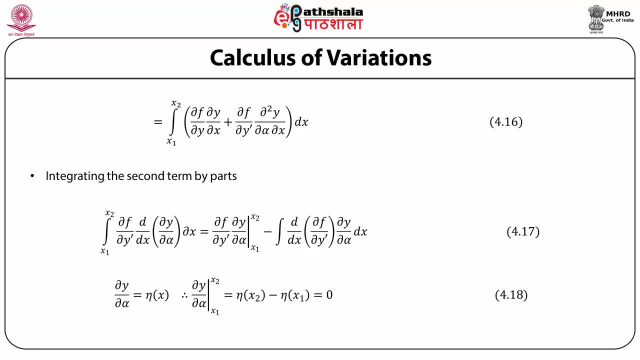 is equal to first function, which is the f by dy prime. integral of the other function is the dy by D alpha, evaluated between the fixed points x1 and x2, minus interior differential of the first is a DDX of df into dy prime, into integral of. 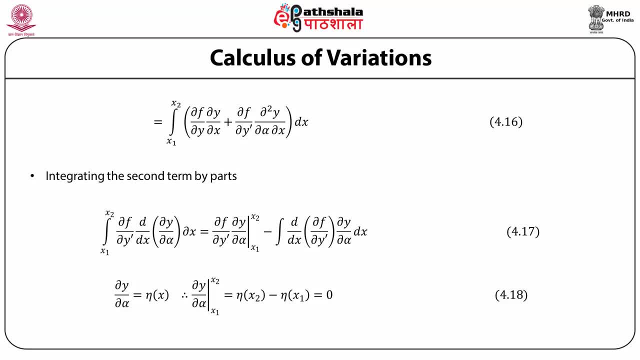 the other we see dy by d alpha integrated over DX. now from the equation, the parts which we have taken: DY by D, x by d alpha is equal to eta x. therefore dy by d alpha between the points x1 to x2 is eta x2. 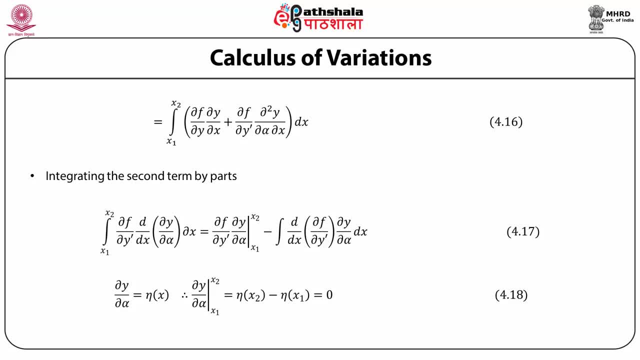 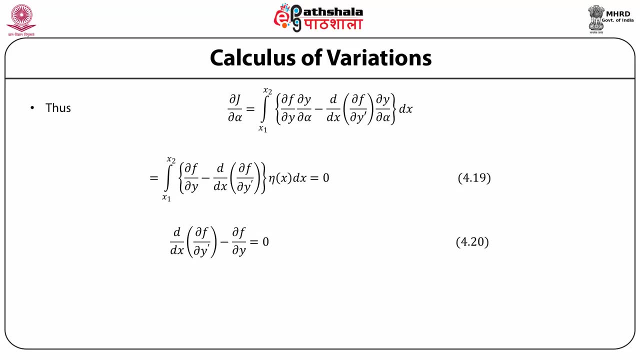 minus eta x1, but the variation at the end points vanishes. therefore this quantity is equal to 0. that means dy by d alpha, when integrated, evaluated between extreme points, is equal to 0. therefore we have d j by d alpha equal to the integral from x1 to x3 of d f by dy, dy by d alpha. 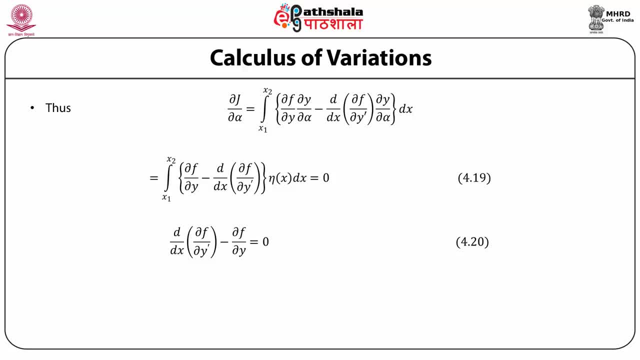 minus d dx or d f by dy prime, dy by d alpha, dx, which is equal to d f, by dy minus d dx of d f by dy prime and dy by d alpha. being eta x into eta x dx is equal to 0, and this must be true for all arbitrary variations. eta x, therefore d dx. 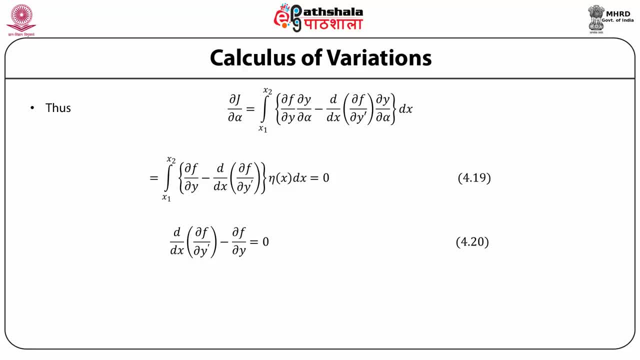 of df by dy, prime minus df by dy is equal to 0. this is an important result. this says that the function to be extremized between the limits fixed limits must satisfy this equation, that is, d? dx of df by dy. prime minus df by dy is equal to 0. this is the euler equation. 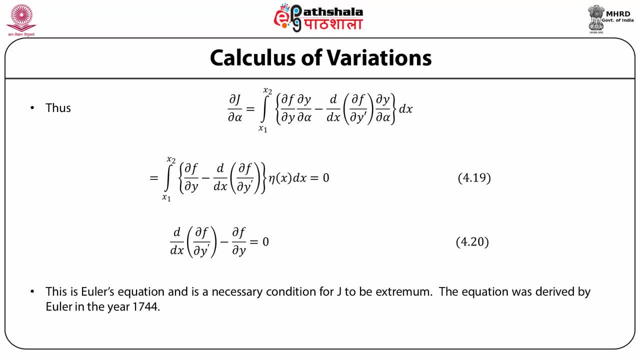 and this is a necessary condition for the functional j to be an extremum. this equation was derived by euler in the year 1744, so remember that if you know the function that has to be extremized, then to the extremum of that function should be such that it satisfies this euler. 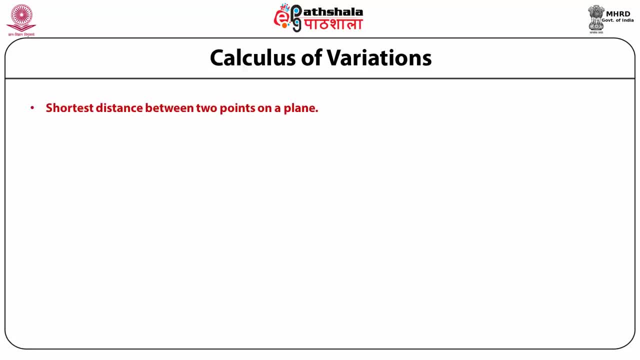 equation. we will illustrate this by simple examples. the simplest example is the shortest distance between two points on a plane. you all know that the shortest distance between two points on a plane is a straight line passing through these two points. this is extremum. now if i take two points, x, y, and a nearby point, x plus dx and y plus dy, the infinitesimal distance. 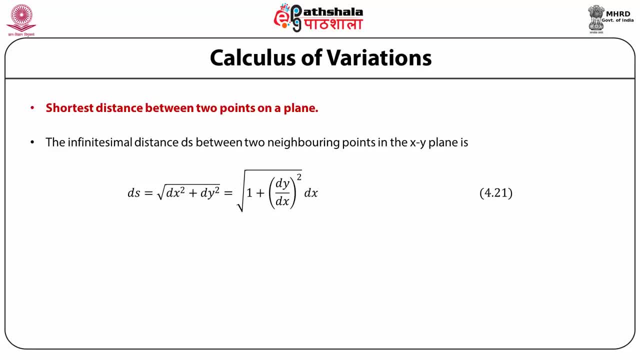 between these two neighboring points in the xy plane is: ds is equal under root of dx square plus dy square which i can write as: ds is equal to 1 plus dy by dx whole square under root into d x. now the total distance between two points a to b is the integral of this. 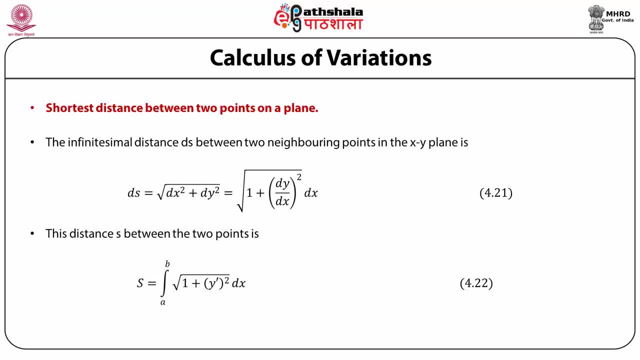 over dx from a to b, that is the distance s is equal to 8, is given by the integral of plus y prime square where y prime stands for dy, by dx, y prime square under root dx between the points a to b. So what we have to do? we have to extremize now this functional s. 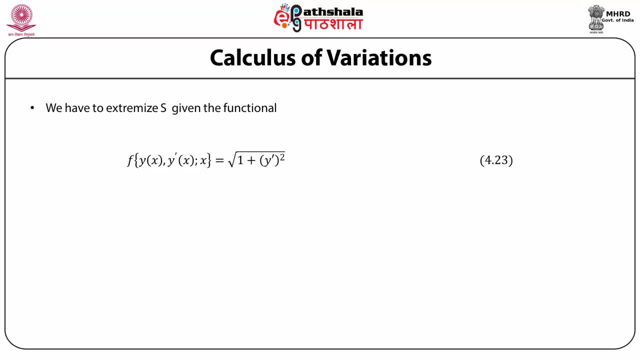 So our function then, which will extremize this, is function of y prime x and x. this is 1 plus y prime, square under root. Now for the extremum of this function. it should satisfy the Euler equation, namely ddx of df by dy. prime minus df by dy is equal to 0.. From the 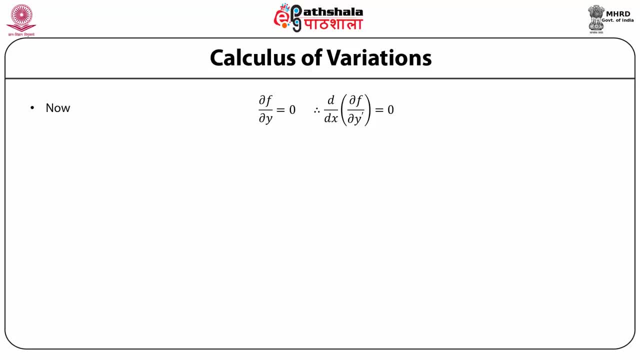 expression of the function f, which is 1 plus y prime. square under root, we immediately see that df by dy is equal to 0. Therefore ddx of df by dy angle y prime is equal to 0.. So f which is 1 plus y prime. 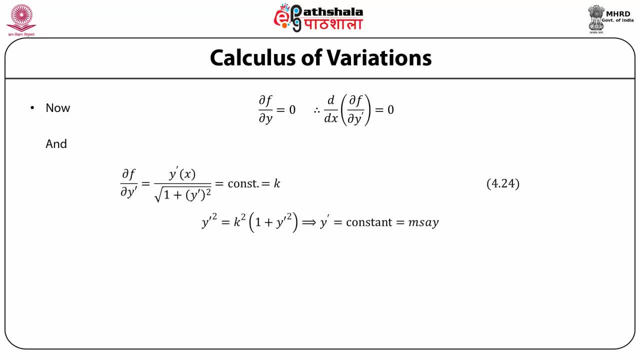 df by dy prime must be equal to 0.. Now df by dy prime is equal to y prime x divided by 1, plus y prime square under root. Now for the derivative of this with respect to x to be 0, this must be a constant k. So we have y prime. y prime square is equal to k square. 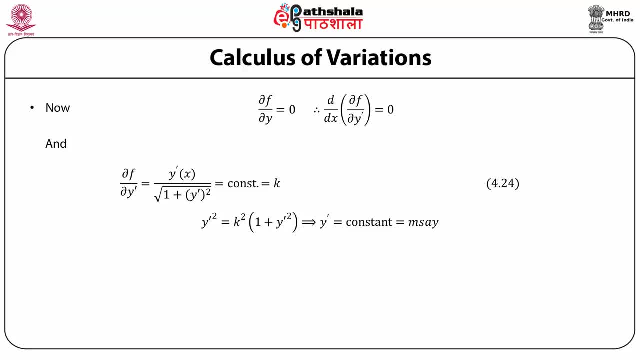 into 1 plus y prime square is equal to this. Therefore, what does it say? It says that y prime is equal to constant. So the solution of this, the y prime square is some k times into 1 plus y prime square, implies that y prime is constant, and which means, when we 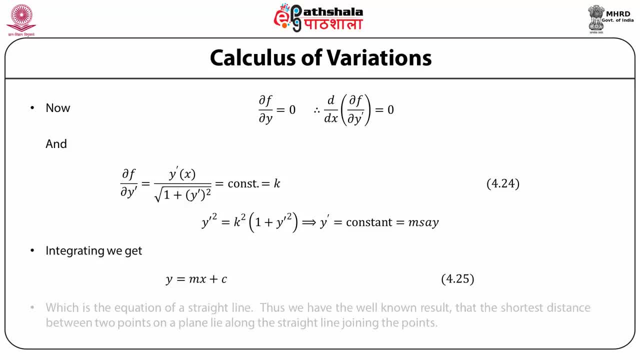 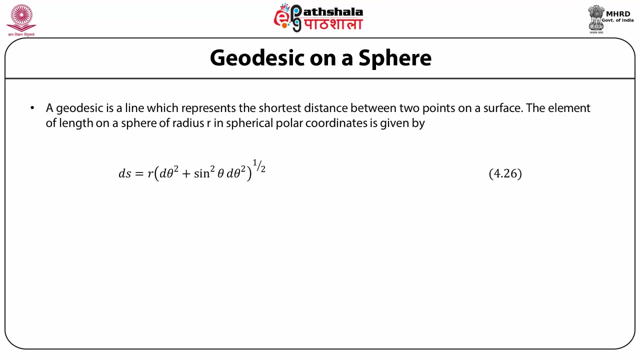 integrate it that y is equal to mx plus c, which is the equation of a straight line, and we have the well-known result that the shortest distance between two points on a plane lies out. We now consider a slightly more difficult problem, that is, of geodesic on a sphere. What 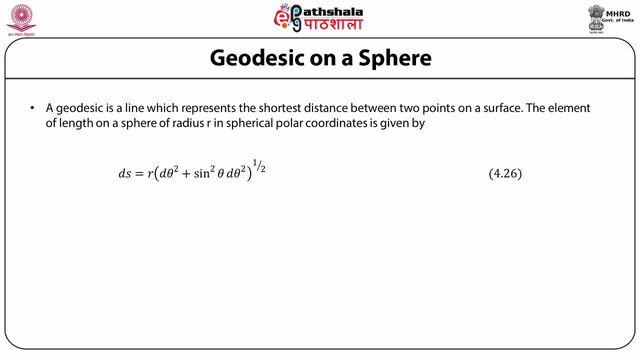 is a geodesic. A geodesic is a line which represents the shortest distance between two points on a surface. In the earlier example we saw that if the surface is a plane surface, then the geodesic is just a straight line. 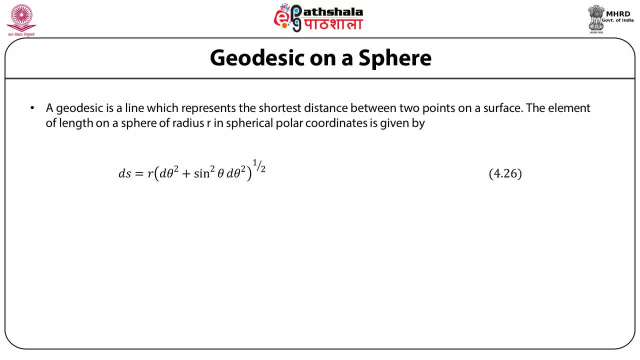 Now we want to find out what is a geodesic. Okay, so what we have found is that if the surface is a square, then the geodesic must be of a size 0. So we need hoping that the very next point of the Law could be of a size c. 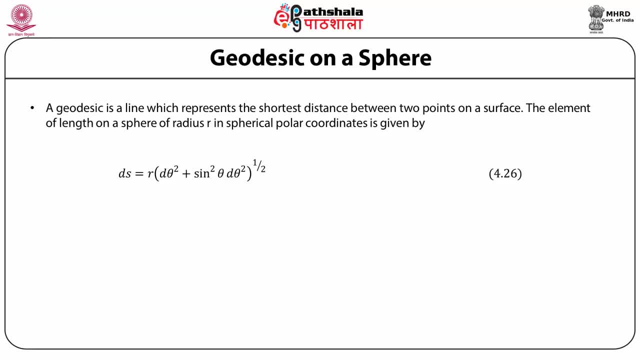 So we will go into Geodesics and we will search for it. Let us first consider the geodesic of a space. Let us look over the sketch, this time the threshold for Rubik�s square, which is 1 s, into 1 pWells. 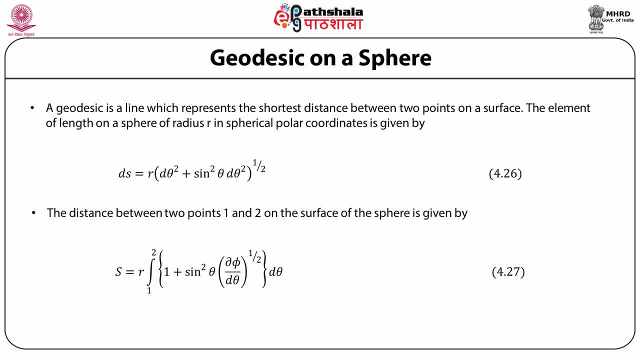 We have 3 esquaries, 1 pp карт at ppretthosquare and we will find the geodesic on the surface of the square is given by: s is equal to r, where r is the radius of the sphere integral from the point 1 to 2 of. 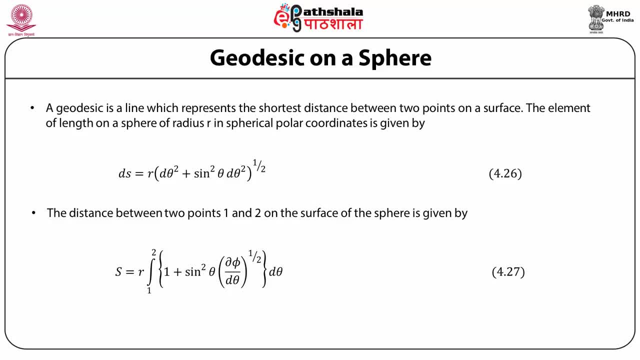 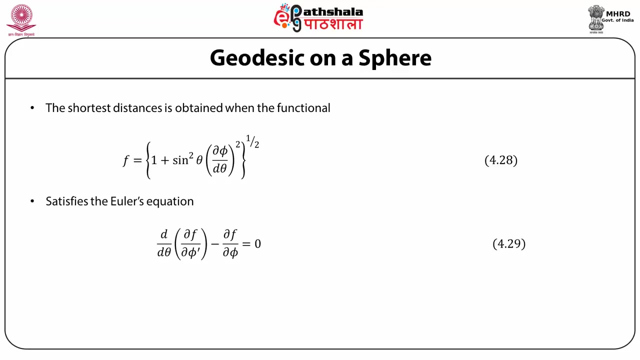 1 plus sine square theta d phi by d theta, whole square under root d theta. So the shortest distance is obtained when the functional f, written as 1 upon sine square theta d phi by d theta, whole square under root, satisfy the Euler condition, namely d d theta of d f by d phi, prime minus d f. 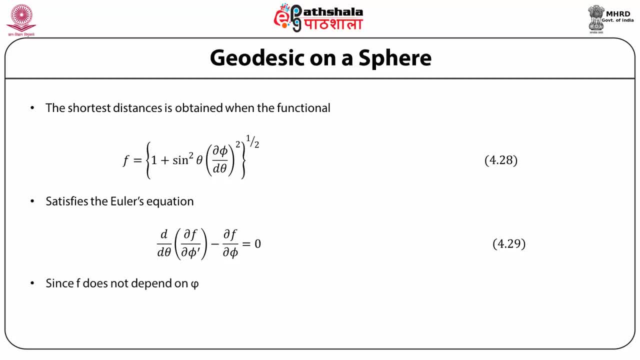 by d phi is equal to 0, since f does not depend on phi. Now d f by d phi is equal to 0 and d f by d phi prime is equal to sine square theta phi prime divided by 1 plus sine square theta phi prime. 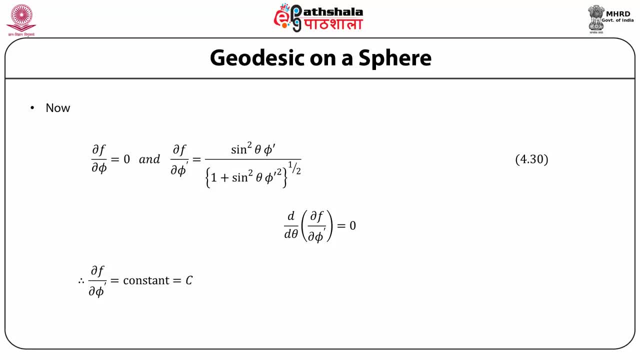 square under root. Therefore, the equation to be satisfied is: d? d theta of d f by d phi prime is equal to 0. therefore d f by d phi prime is equal to constant. and let us put that constant to be equal to c. Then, substituting in the equation above, then we have: 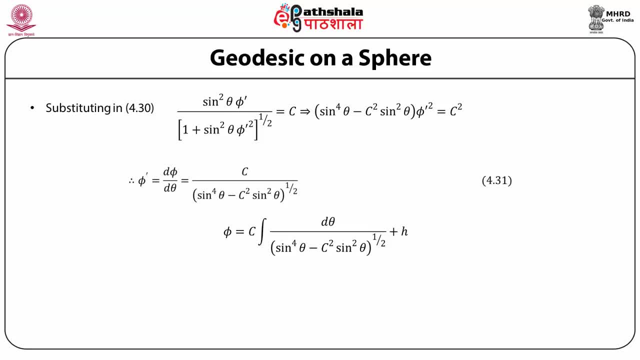 sine square theta. phi prime divided by 1 plus sine square theta, phi prime square under root is equal to a constant c which can be solved for phi prime, and we get phi prime which is defined as d phi by d theta is equal to the constant c divided by sine 4. theta minus c square sine square theta under root. 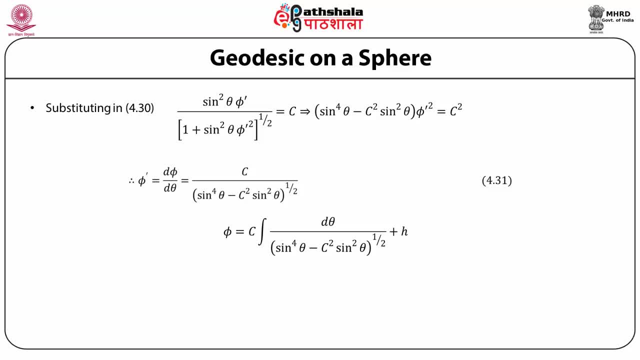 Therefore phi is the integral of this plus some constant h. The integral can be performed without much difficulty By substituting t for c의 pour theta, in which case d? t is equal to c cosine squared theta d theta and therefore phi. in this variable, t can be written as: or is given by: phi is equal to c into d t divided by 5 c. 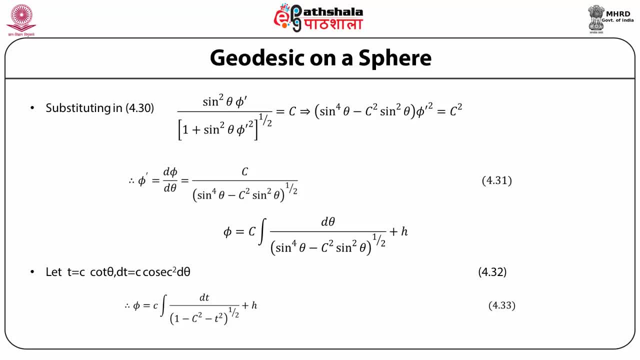 equal to c into d, t divided by minus c squared, minus c square under root, plus the constant h. Now this method can be looked at in other forms. this was the 베immeter fundamental squares, guess, I will call it the formulae output. there is one more way you can simplify the question: is called a 점ert adventure- apostrophe-. 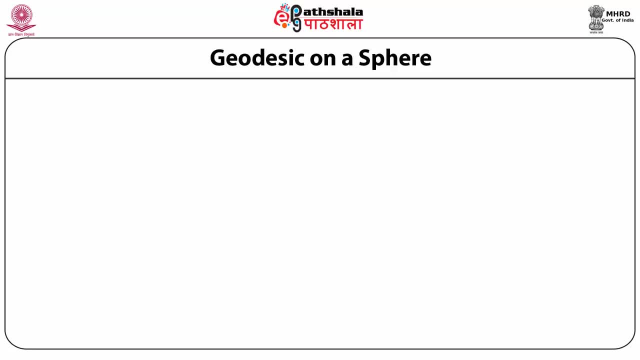 but we have done all while taking this further. that is, areascinação esprite. Now, because i have written the equation for d, thetaI and derf is taken care. suffer by this. Now this can be easily integrated and we get: phi is equal to c sine inverse t by b plus. 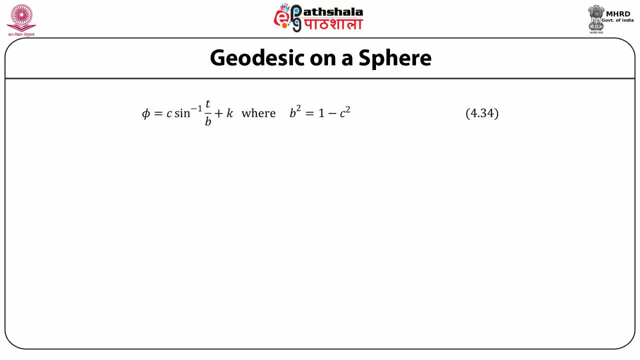 k, where b square is equal to 1 minus c square, which can be written as b sine of phi plus k, is equal to k, is equal to c cot theta. Therefore, cos theta is equal to b sine theta sine phi. cos k plus b sine theta. cos phi sine k, where we have expanded sine phi plus k as sine phi. 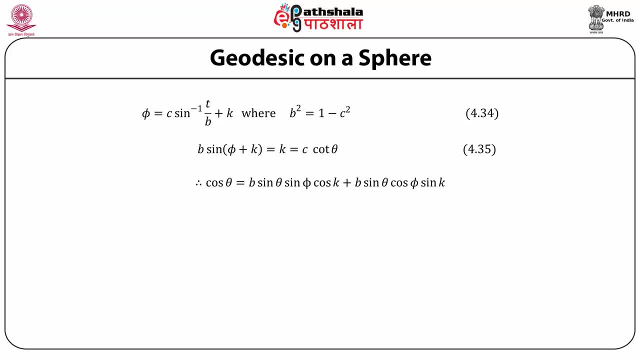 cos k plus cos phi sine k. Now, if you multiply this by r, we have c r cos theta is equal to b cosine k of multiplied by r sine theta sine phi plus b sine k multiplied by r sine theta sine phi, Substituting for r sine theta sine. 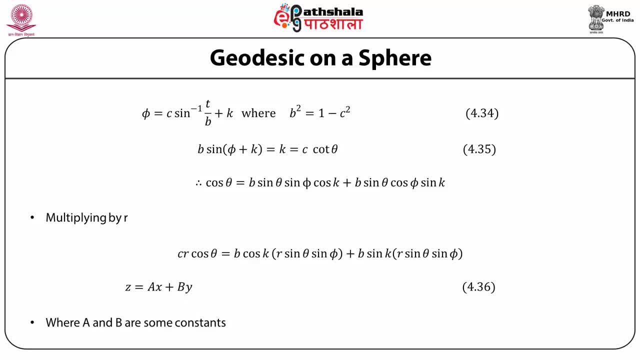 phi and r cos theta sine phi, in terms of the Cartesian coordinates, and r cos theta being equal to z. From this we get that z is the moment when a and b and z square SPD. That has to be expressed as as follows: Here: r is the moment and the bundled agreed points of this equation is the moment of times. 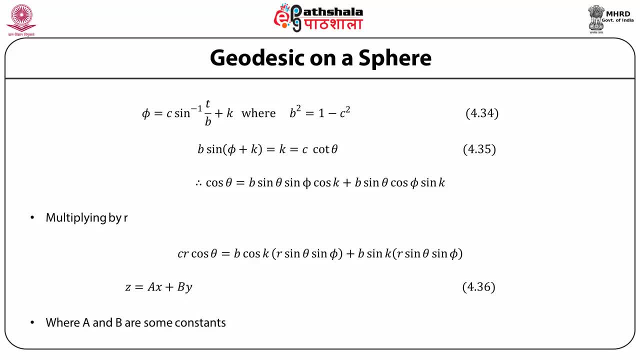 0. So out of this we get that we must get the engineer equation that gave a transform mice. The equation we get is: z is equal to ax plus by y. That is first we consider the problem in this vehicle. polar coordinates after carrying out. 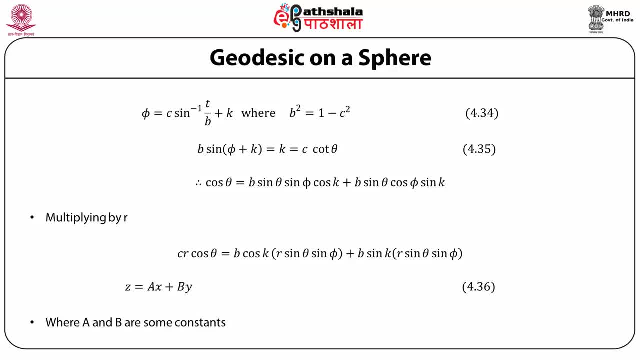 the integral To see what kind of a geodesic we get. we are reverted back to the Cartesian coordinates and you get the equation for the geodesics, as z is equal to ax plus by Y, where a and b are some coordinates, b are some constants. Now can you recognize what kind of a curve is this? or what is this? 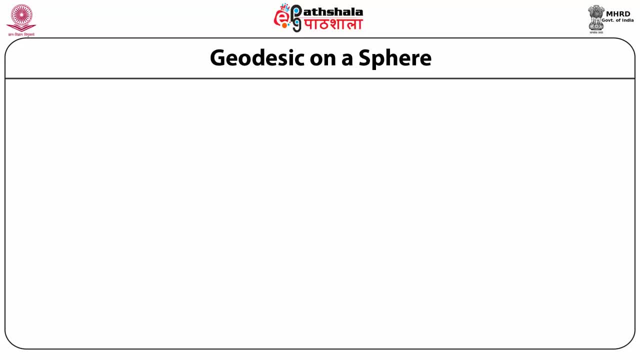 is a curve, a surface or plane whatever. Now you can see that this is the equation of a plane which passes through the center of the sphere, because x is equal to 0, y is equal to 0, z is equal to 0 is a solution of this. So you have the geodesic, such that you have a plane passing. 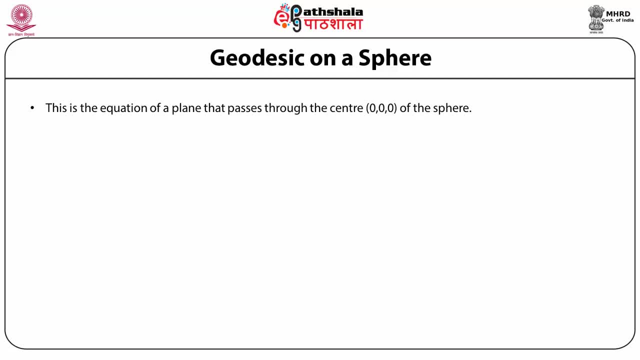 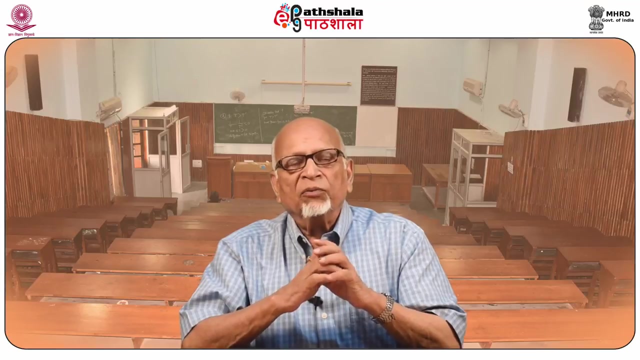 through this center of the sphere. Now, this plane cuts the surface of sphere on a circle, and this circle is called the great circle. Thus, the shortest distance, that is the geodesic, between two points of a sphere, lie on a great circle. passing through these points, We will now consider what is known as the 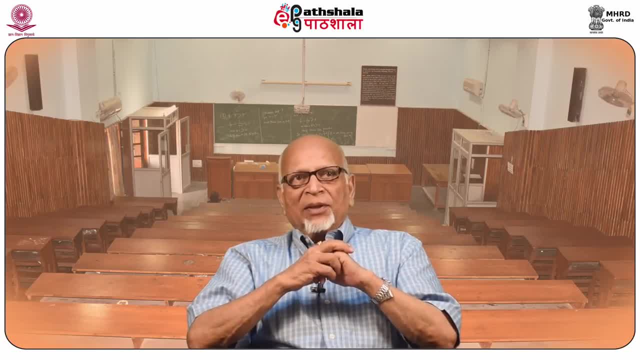 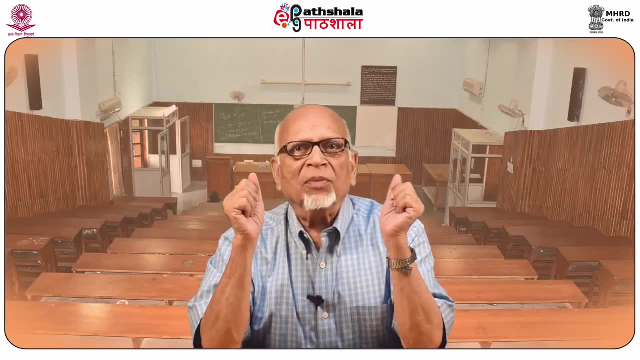 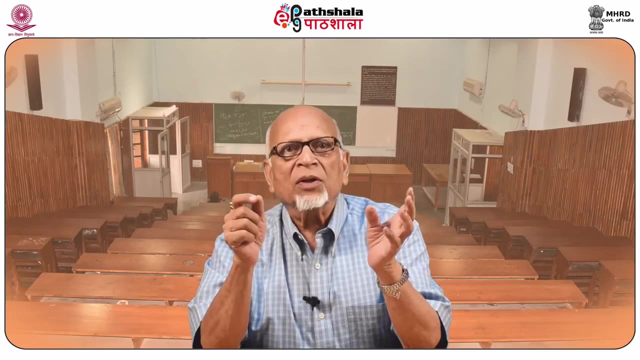 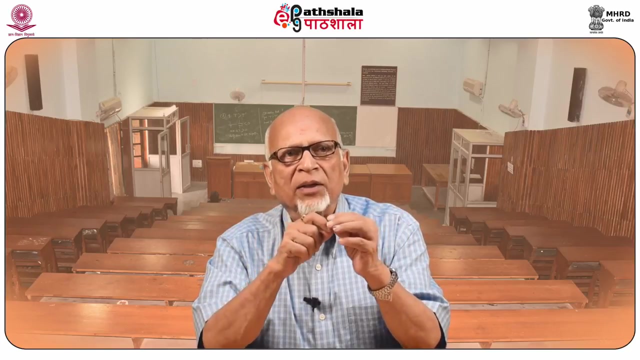 brachistochron problem. This is one of the classical problems in the calculus of variations. This problem is to find the path on which a particle moves in the presence of a constant force, as to make the term. It is the time taken by the particle to move from an initial point to a final point minimum. 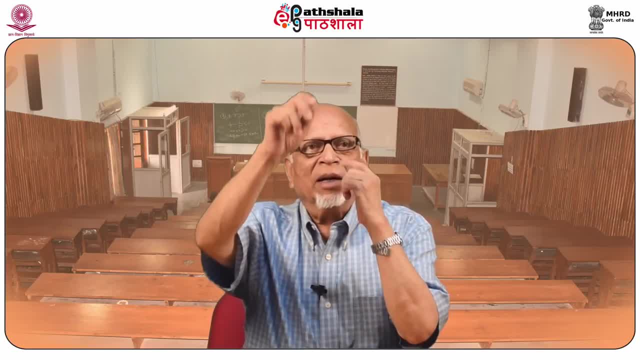 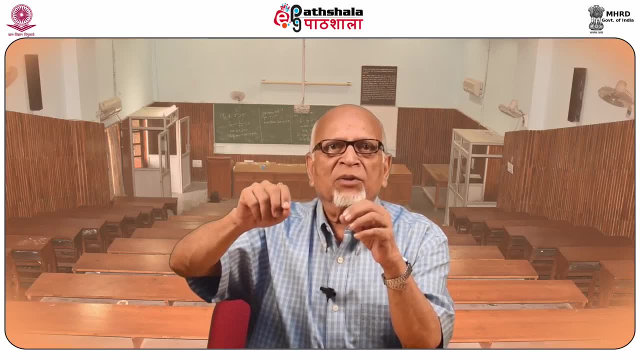 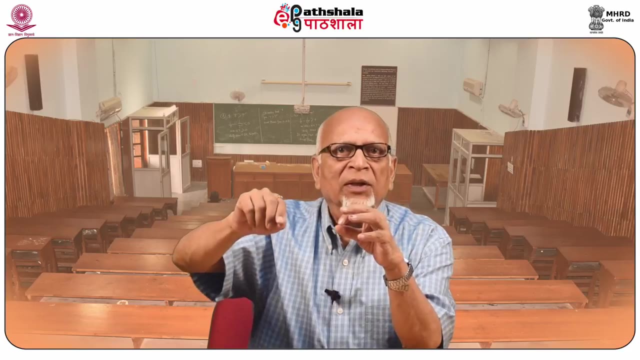 For example, if the particle falls under the force which, if you take to the gravity, then the problem is to find the path. Then what should be the curve on which the particles moves under this constant force of gravity which will make the time taken from thatfilter down to the final point minimum? This is called the brachistochron problem. 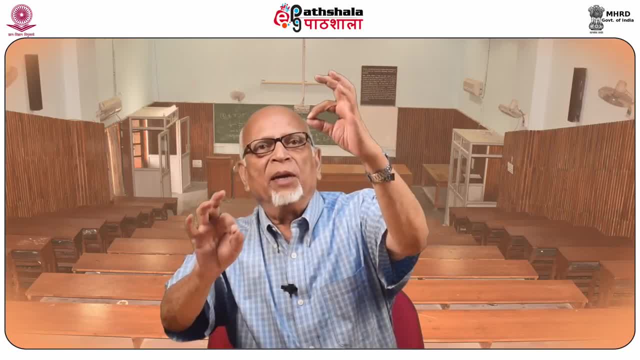 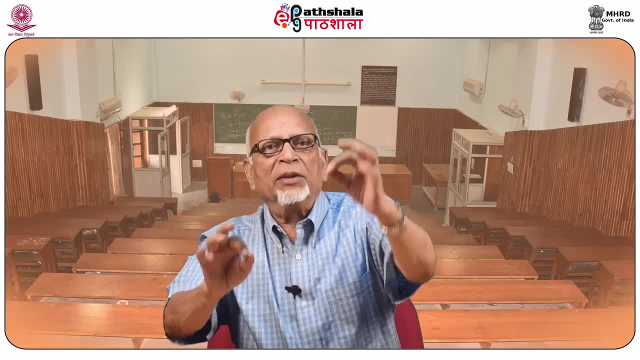 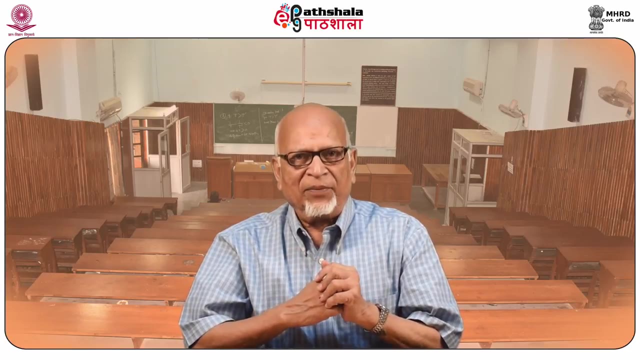 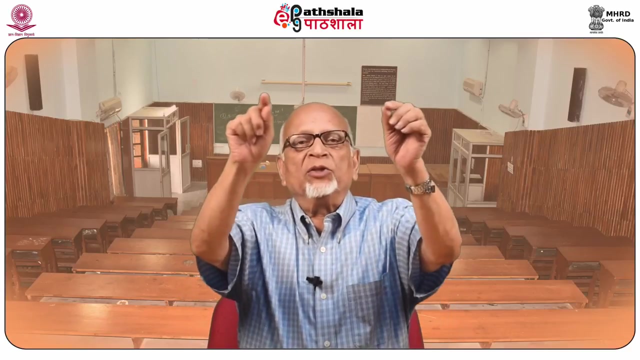 taken by the particle from point A to point B, a minimum. So this was a problem which is known as Bracastrocon problem and this problem was first solved by Johannes Bernoulli in the year 1696.. To solve this problem, we will choose a coordinate system. So we choose. 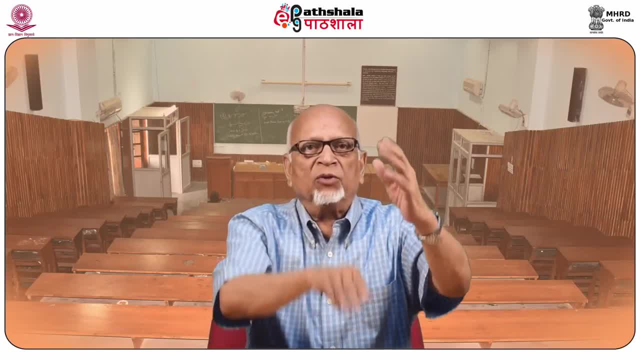 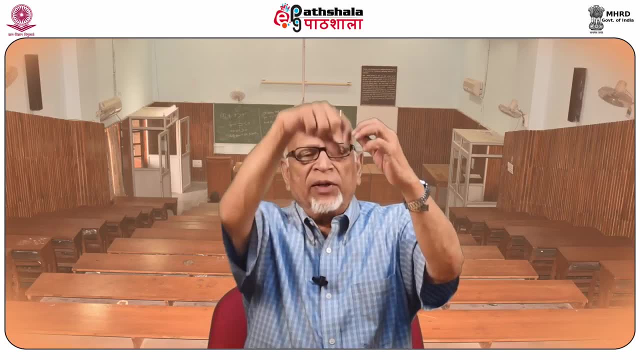 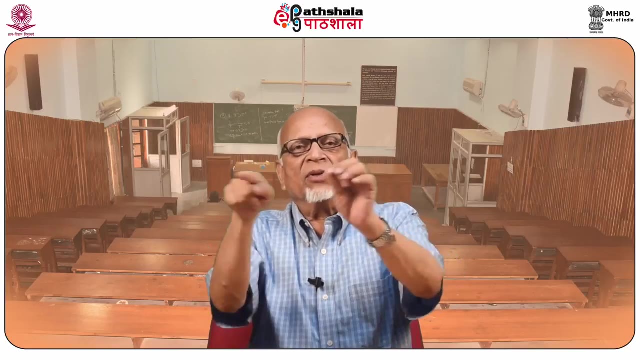 a coordinate. the particle moves on a curve, So the curve is on a plane. So we choose a coordinate system So that the initial point lies on the origin and the force field is directed along the positive x axis and the other axis, or the y axis, with the horizontal 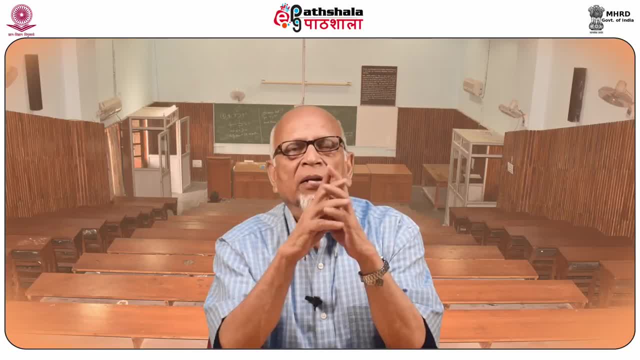 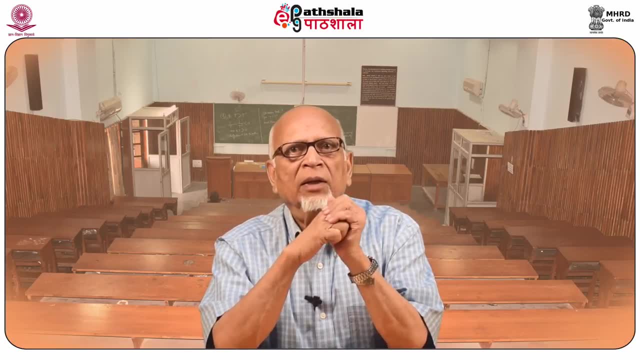 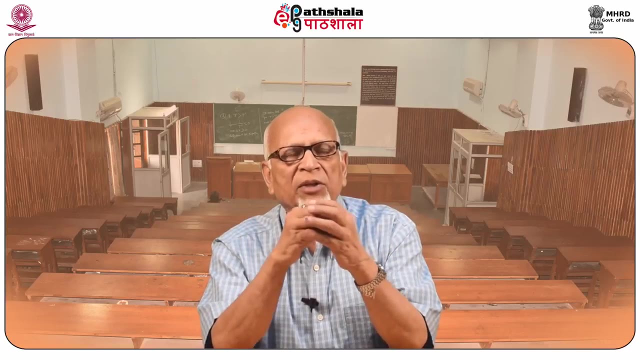 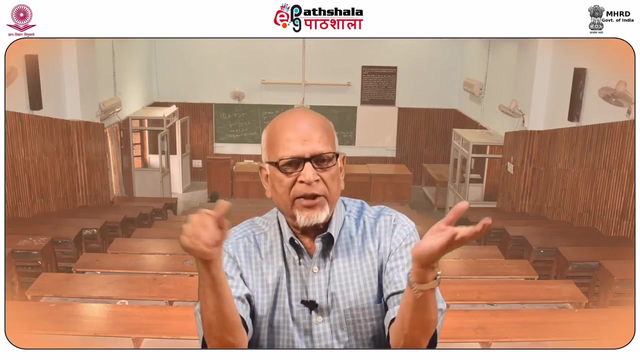 axis, We assume that there is no force of friction and there is constant force of gravity acting on the particle. The force of gravity is constant, which is m times g, where m is the mass of the particle, The total energy of this system during its transit. 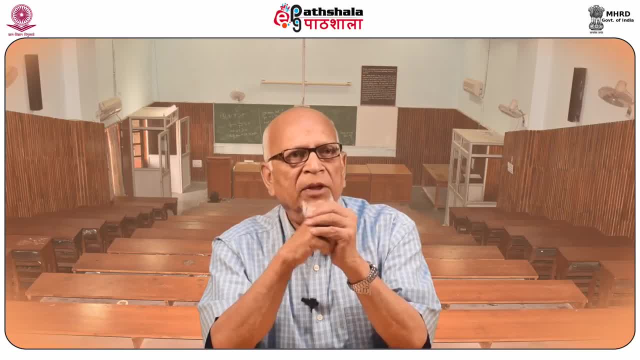 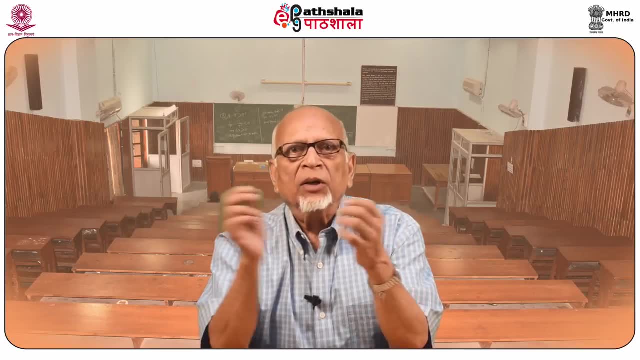 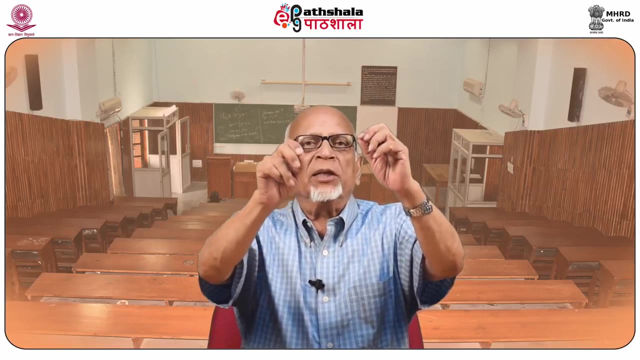 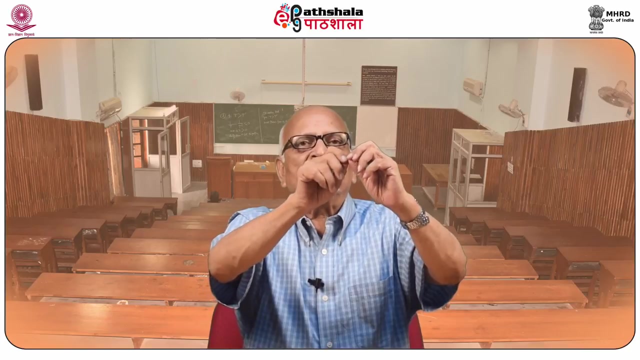 is conserved because gravity conservative force, That means the total energy, which is equal to sum of the kinetic energy and the potential energy- must be constant. So at the initial point we take the potential energy to be equal to zero and the particle starts at rest. So it is. kinetic energy is also 0., So t plus u is equal to zero at the initial. 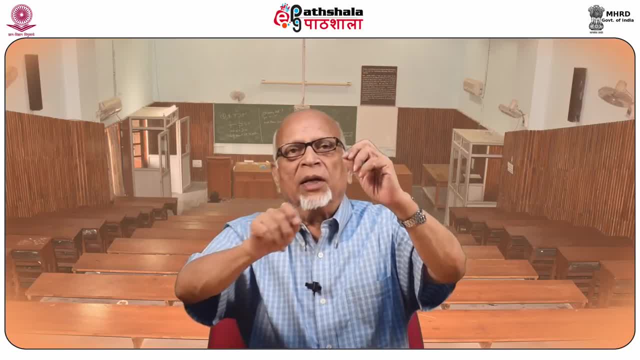 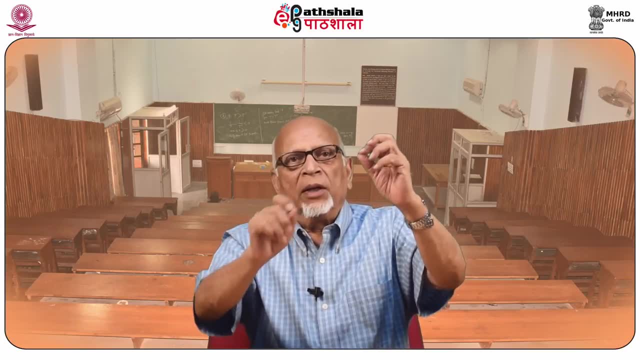 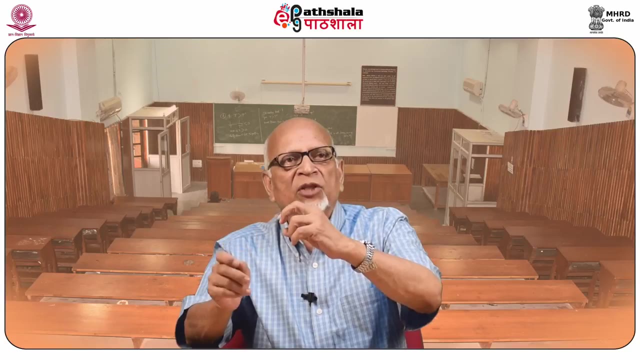 point and and. as the particle moves along this curve, and since the energy is conserved, the total energy remains equal to 0.. So at any point in the transit, the kinetic energy is half mV square and the potential energy is minus Mg x, if x is is the coordinate of. of of of the particle approaches. top of there is a visual Nobody 중 g. This is h spent equal to E by m x 1,n δ. So this is got to be zero. Therefore the energy of VICts will go. B equals to labsed. So the curl of the lobes is: maintain my equation of: I divided by 6 units. 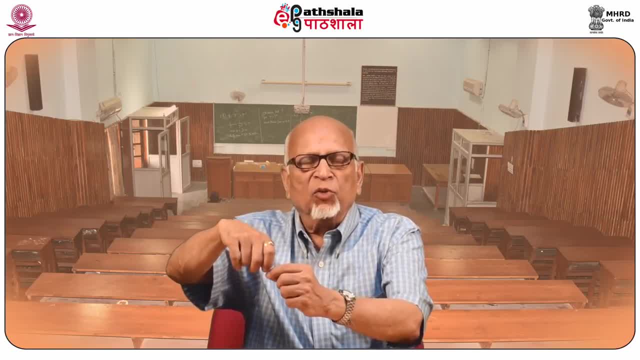 C is equal to 1n muv, So the normal Gonna be minus mу I or m by 2 m Get the quasi-vewl of energy which is equal particle which is moving along the direction of gravity. So half m v square minus m g. 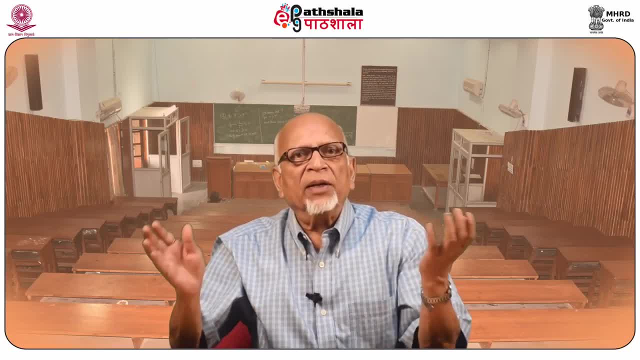 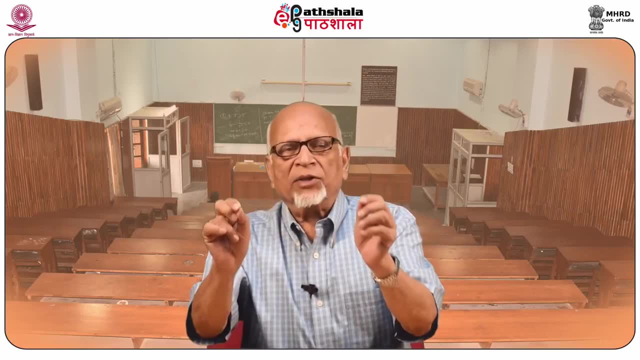 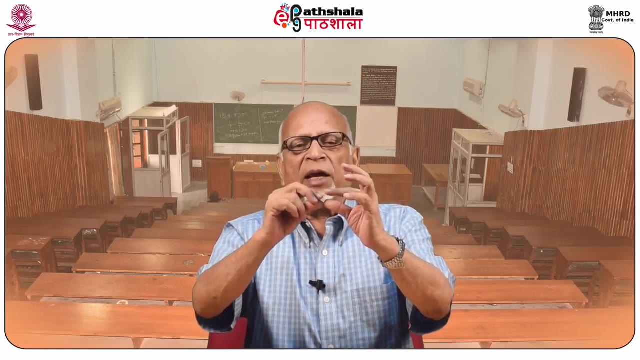 x equal to 0. that means the velocity of the particle at any position is given by under root 2 g x. So we know the velocity. we know the velocity at any point. So what we do? we take a small line element and find out how much time is taken to travel the distance. 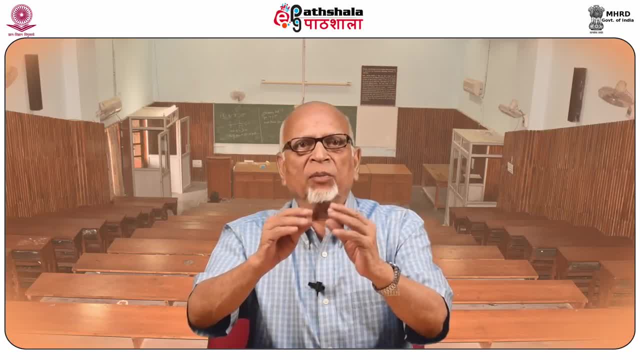 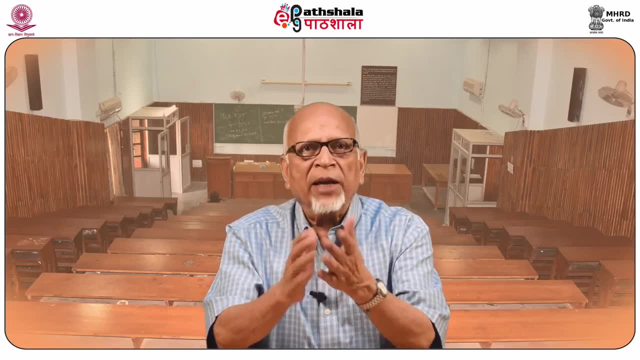 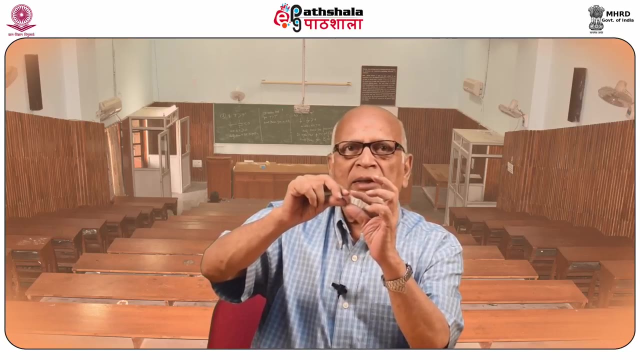 So the time taken by the particle to transit from the initial point to the origin x, y, we will write down. and so this time is suppose we take two neighboring points, then the line element is given by d s, So the time taken by the particle to traverse this distance. 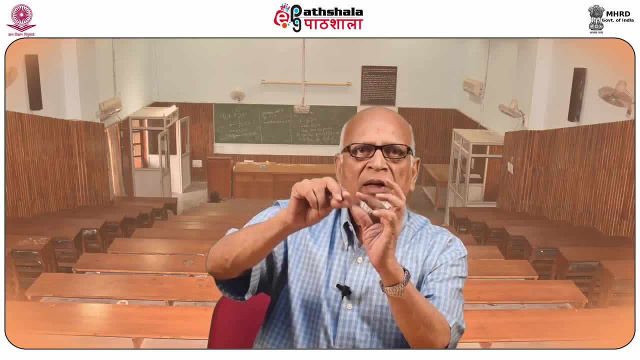 d s is equal to d t, which is d s by v and d s. the line element is a d x square plus d y square Under root, and v is equal to under root 2 g x. So d t is simply equal to under root. 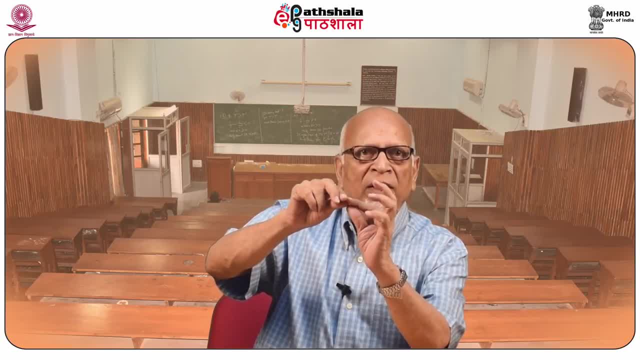 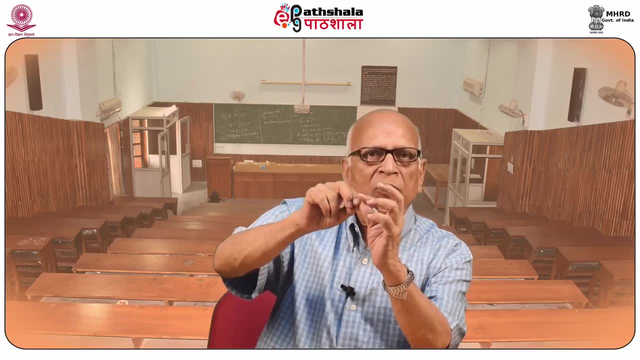 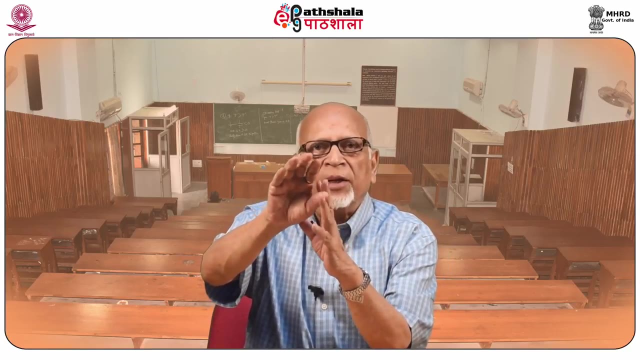 d x square plus d y square divided by v, integrated from initial point, which is which we are taken the origin, 0, 0, to the final point x, y. So the time taken then is represented by this expression: 1 by root, 2 g under root of 1 plus y prime square by x. Now, what is this expression of d x crumbs into the next condition of this equation: D x 1 by the value of k x 😅1 torr bacteria g 0 of t or-ored Plus. to do this you have. 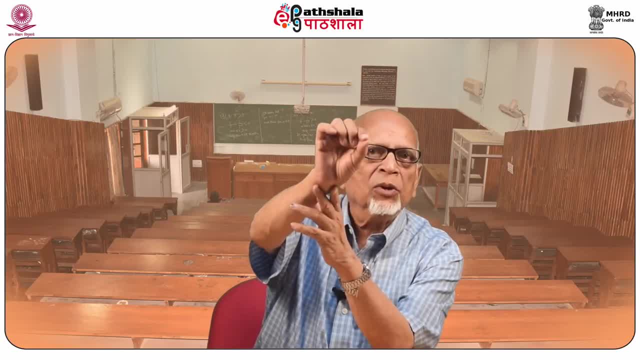 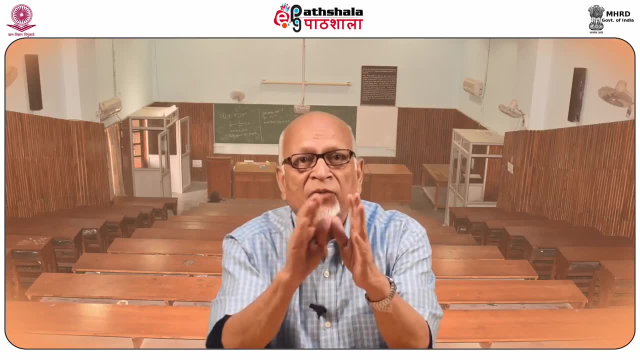 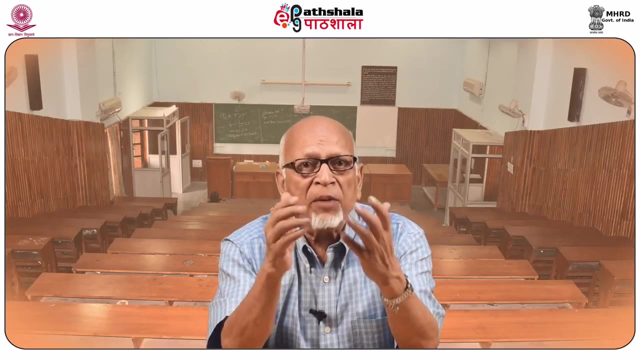 to provide the enriched preventative constant negativebilities 0, 0, p and 1, 0. d, x is equal to now this part m, So that is from the becomes the function which is the integrant, So the function f, which is equal to 1 plus. 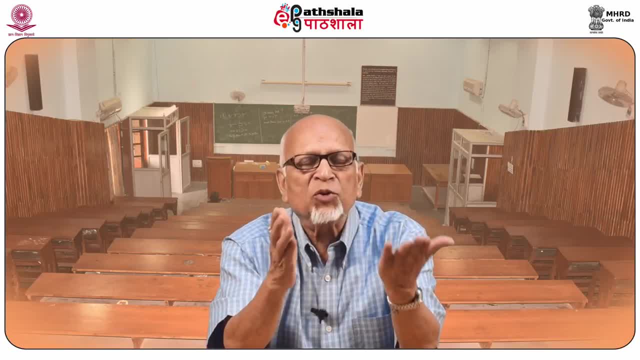 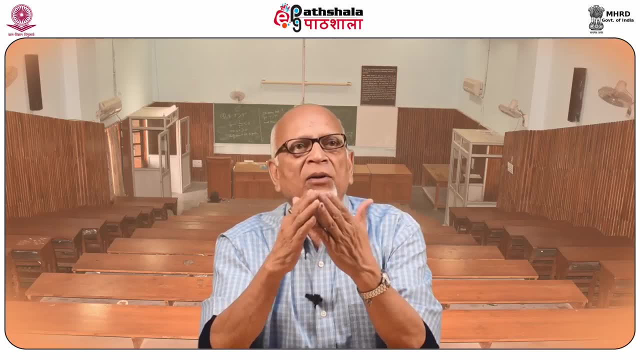 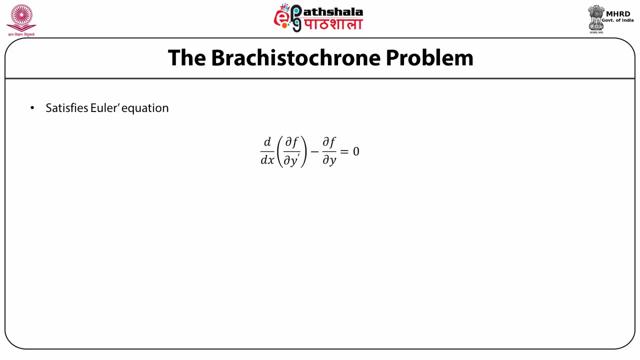 y prime square by. So an Bakers- verdade by x under root has to be extremized. So that's all that we have to do. That means this function has to satisfy the Euler equation for it to be extremum, Continuing with the Barakis-Trikhon problem, that is, the problem of finding the shortest. 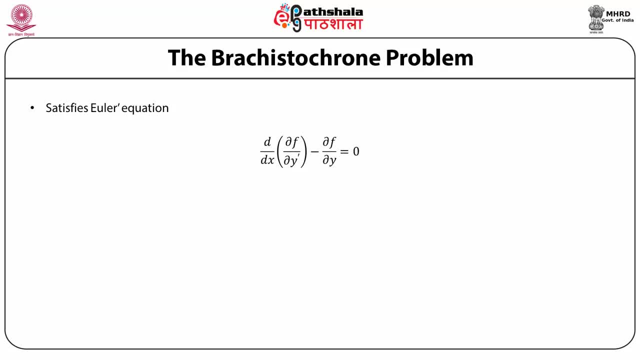 path we have the function f which is to be extremized. The function f was given as equal to 1 plus y prime square by x under root. So this function f should satisfy Euler's equations, which means d, d x of d f by d y. prime minus d f by d y is equal to 0.. The 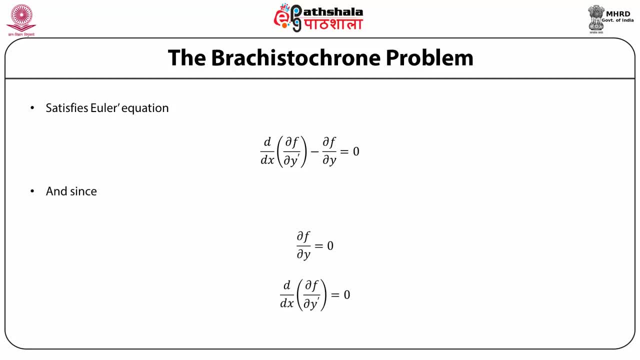 function f does not depend on y, so d f by d y is equal to 0. Therefore we should have d d x of d f by d y prime is equal to 0.. Now d f by d y prime is equal to y prime upon. 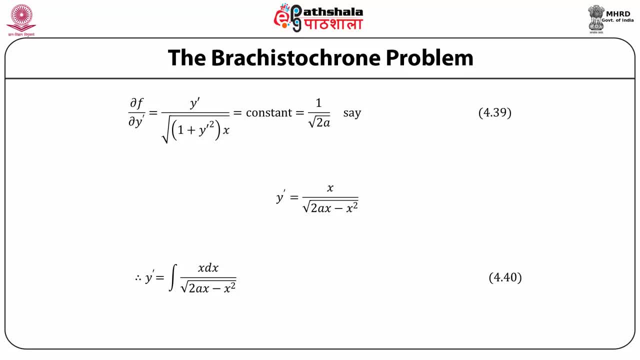 1 plus y prime square by x under root- Thank you- into x under root. and since d d x of d f by d y prime is equal to 0, then this quantity d f by d y prime is a constant. So let us call this constant 1 by under root 2 a. that means y prime. 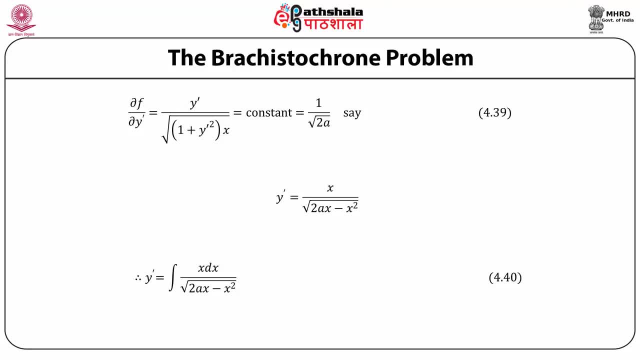 we can solve this for y prime and we obtain: y prime is equal to x upon under root 2 a x minus x square. therefore, y prime is equal to integral x, d x divided by under root 2 x minus x square. to evaluate this integral, let x is equal to a times 1 minus cos theta. then d x is evidently. 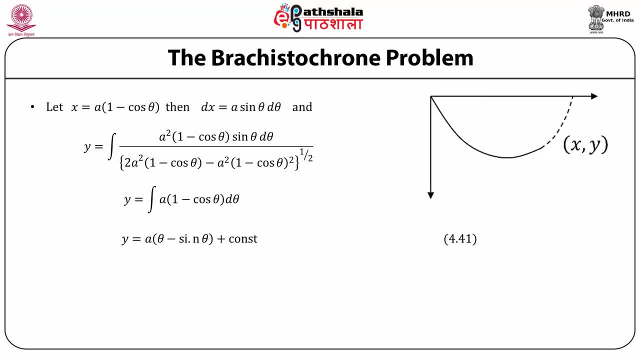 equal to a sine theta d theta. therefore y becomes equal to an integral of a square into 1 minus cosine theta, into sine theta d theta, divided by 2, a square 1 minus cos theta, minus a square 1 minus cos theta, whole square to the power half. So we get from here y is equal to integral a. 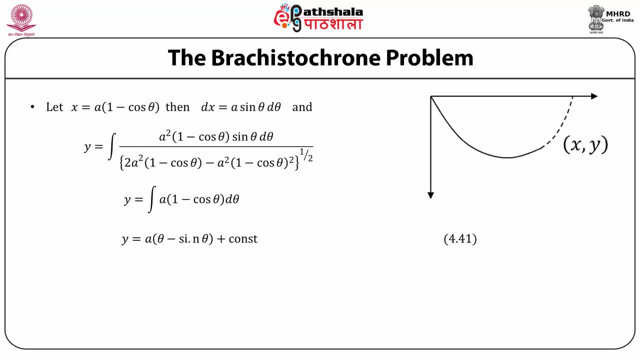 1 minus cos theta d theta which can be integrated, and y is equal to a theta minus sine theta into a constant. So the path taken by the particle to decide between two points the shortest time is given by. y is equal to a times theta minus sine theta plus a constant. 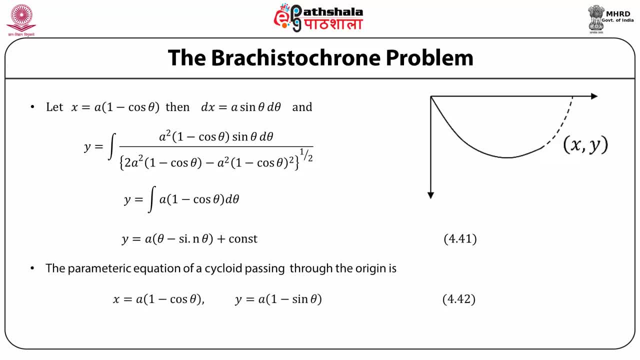 Now the parametric equation of a cycloid passing through the origin is: x is equal to a times 1 minus cos theta, Then y is equal to a times 1 minus sine theta. thus the curve taken by the particle lies on a cycloid as shown.